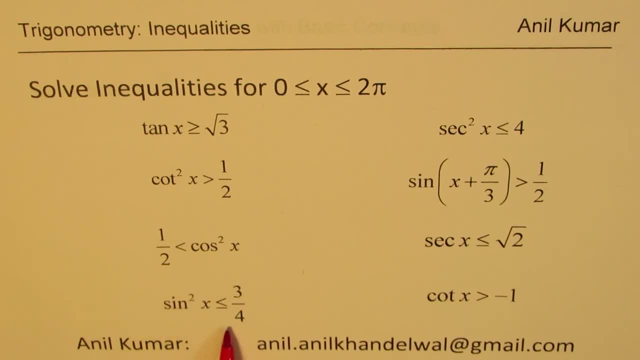 when half is less than cot square x, when sin square x is less than equal to 3 by 4, and some more questions on this side. Now feel free to write your comments, share your views and if there are any suggestions or questions to be answered, you can always send. 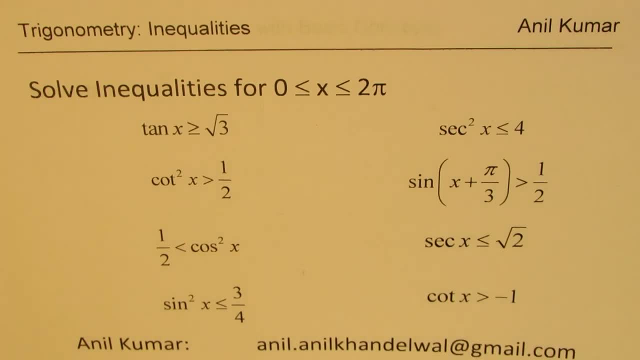 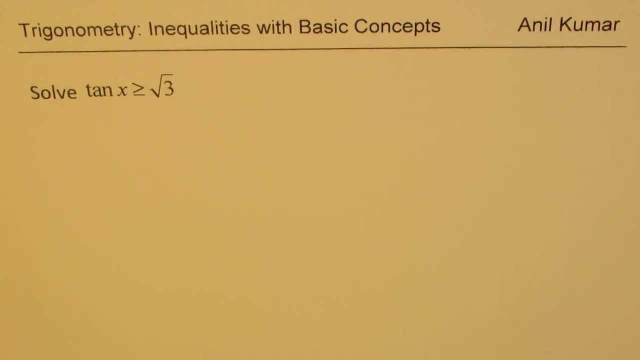 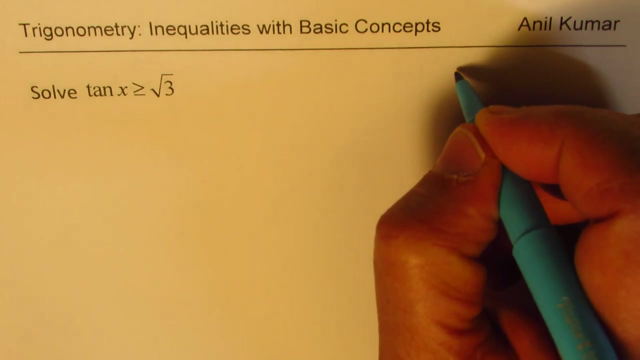 me an email on the address given. Now let's take these examples one by one. Let's begin with tan x greater than equal to square root of 3.. Now here I will actually take the most simple approach, the simplest of all, to solve all these questions. And 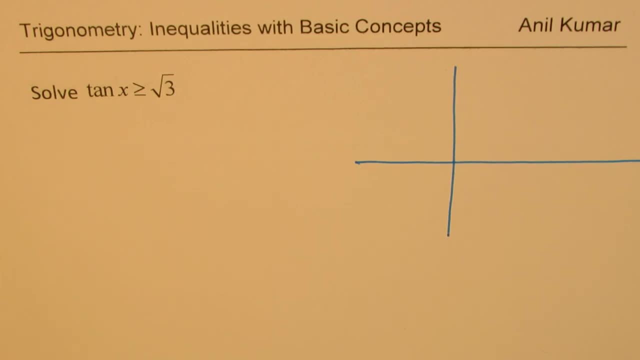 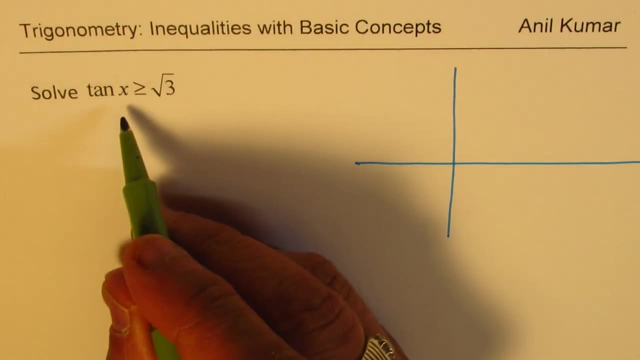 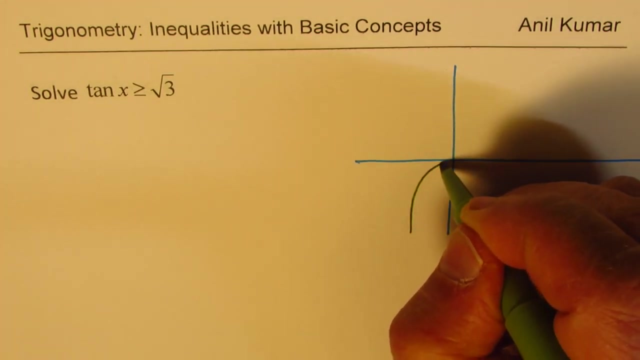 what we are going to do here is look into the graph of the function to get an idea what the solution should be Now. tan x. Tan x has a period of pi, 180 degrees. The graph could be sketched kind of like this, right? So I'm making very rough sketches here. but 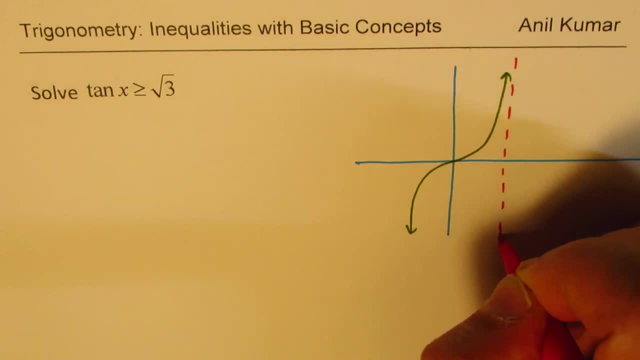 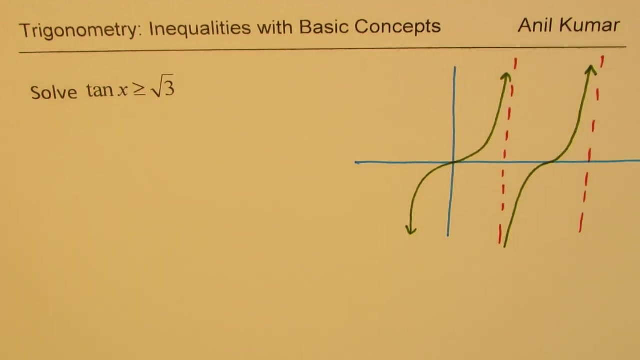 they help us to provide the correct solution. So that is the whole idea. So let me just sketch the tan x function. It will look like something like this: right, So we have drawn two waves. It goes from minus pi by 2 to pi by 2, right, So these are your zeros. So first zero is: 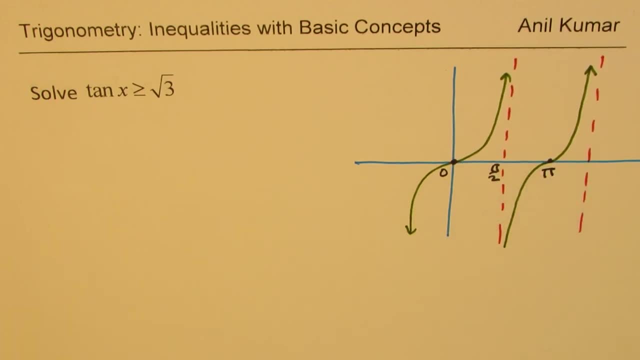 at zero, the second one will be at pi, and then the third one will be at 2 pi. So let me just sketch one more cycle here. Okay, Now these zeros correspond to the sine x value of zero right. Tan is sine over cosine, So 0 pi and. 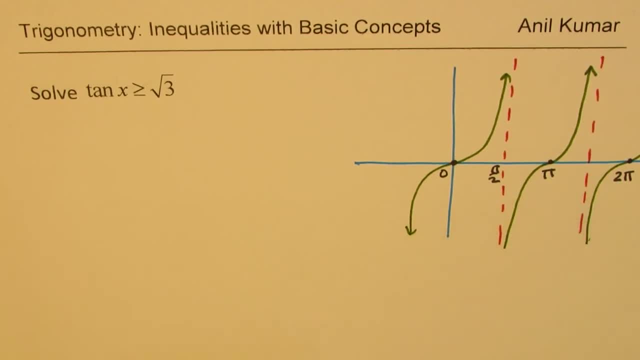 2 pi gives you three zeros for tan x. The inequality which we are trying to solve. is tan x greater than square root: 2. So when a tan x greater than square root: 2. So when a tan x greater than square root: 2. So when a tan x greater than square root: 2. So. 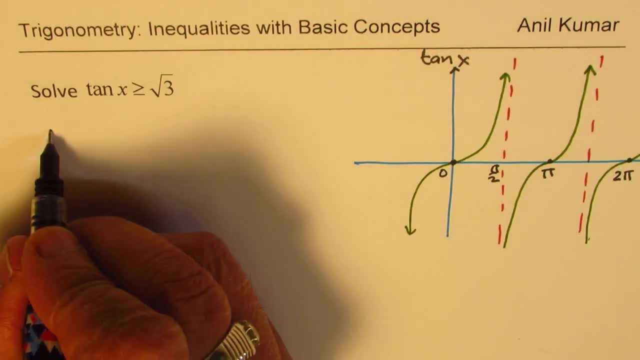 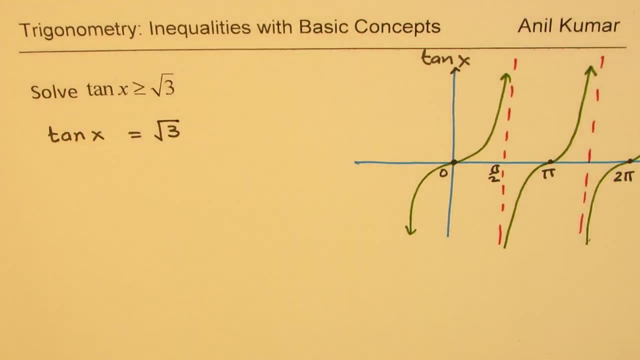 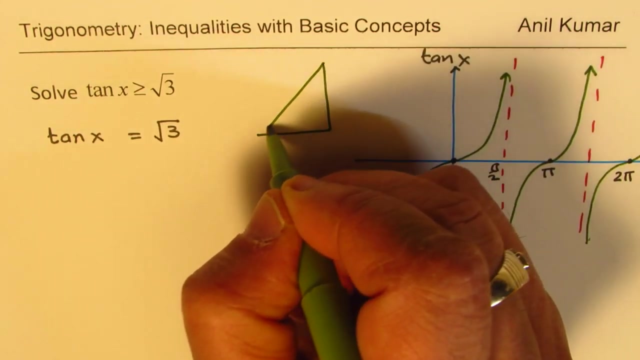 whenever you have inequalities, you should also think about first: what is the value of x when tan x is equal to square root of 3, right? So when you think about this, you will also remember the special triangle which gives you the value of square root 3.. Now 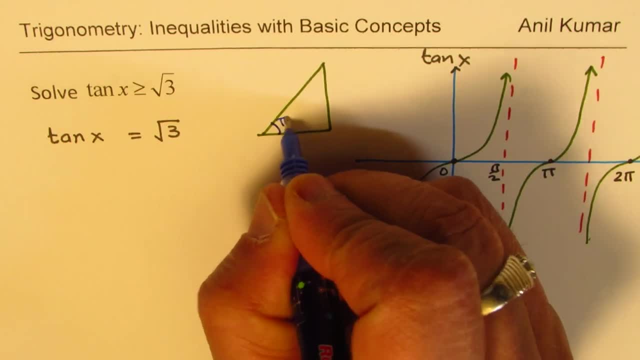 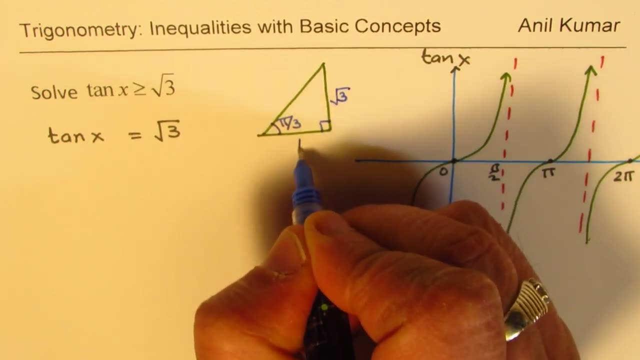 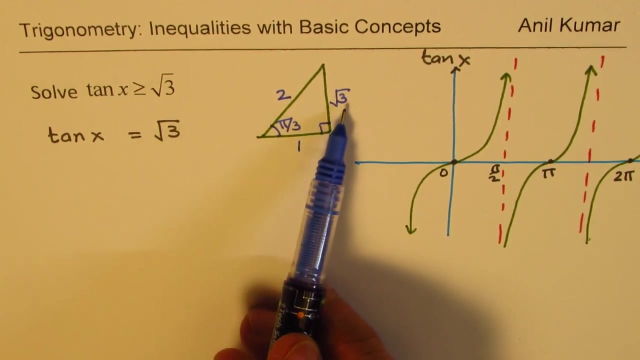 it is 30,, 60,, 90, or pi by 3, angle, which gives you tan of square root of 3, right, And that is your special triangle. So you know that tan x is actually equal to square root of 3, for x equals to pi by 3.. So what we do here is: 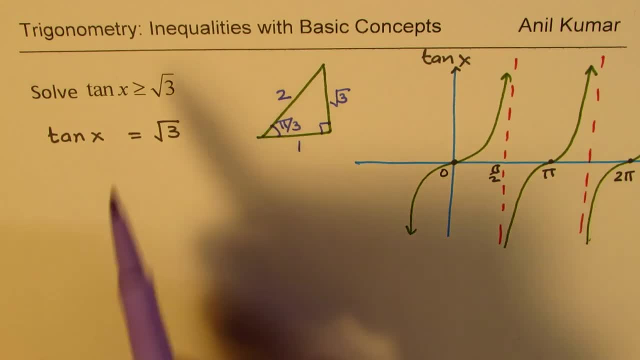 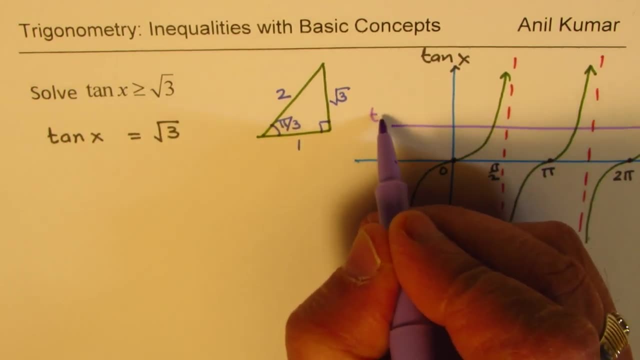 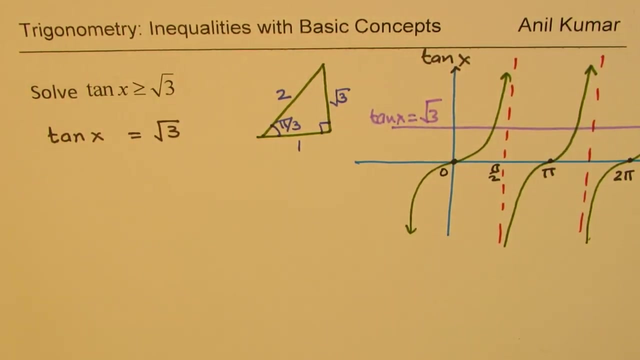 we want that tan x value to be greater than this. So let us say: this represents the value for tan x equal to square root of 3.. So our solution, our solution, lies when the graph is greater than that. right, So that is what we are. 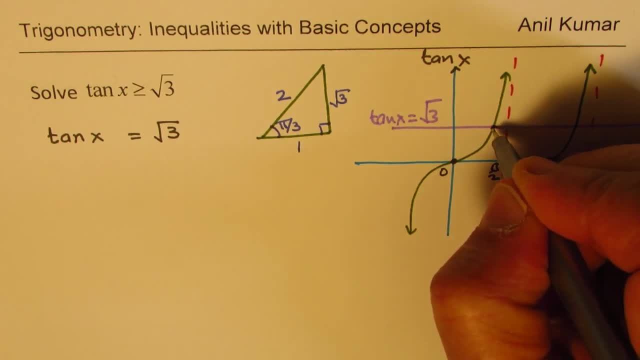 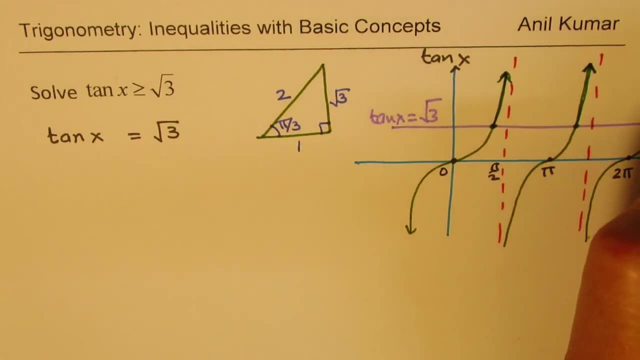 looking for. So that is to say, that is our solution. Greater than equal to means. these points are included, and we are looking into this part of the graph. Is that clear to you, right? So we are looking into this part of the graph. 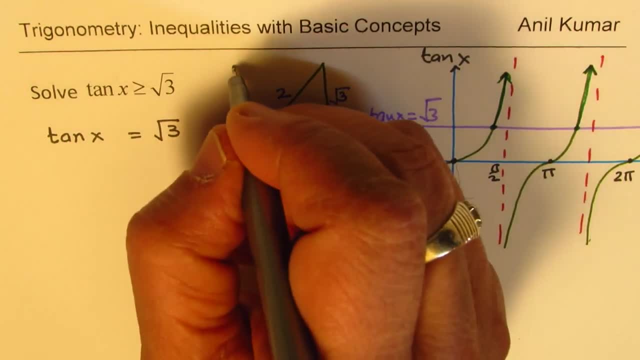 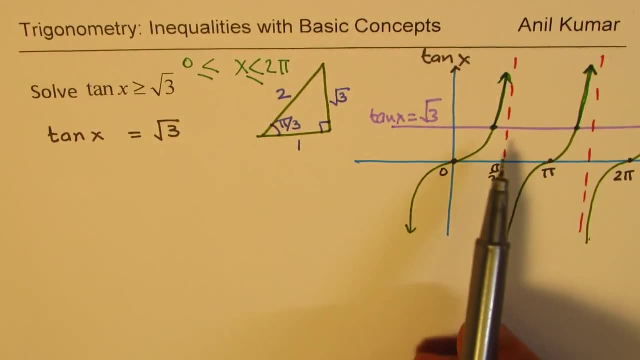 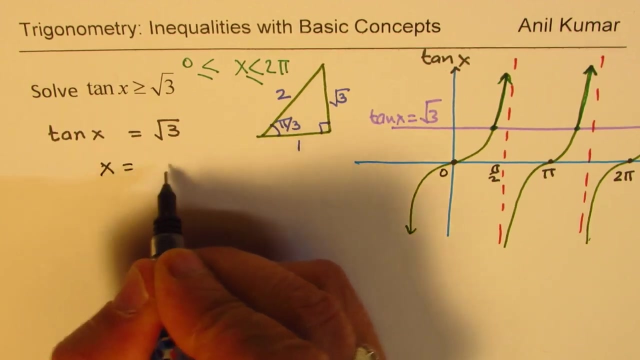 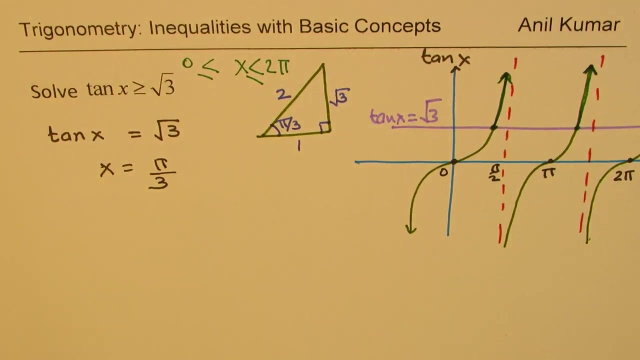 So within this domain, which is from x greater than equal to 0 to 2 pi, we can clearly see the solution is what Do you get the idea right? So from here, we know x is equal to, you know, pi by 3.. Now one more thing will help you to solve these questions, and that 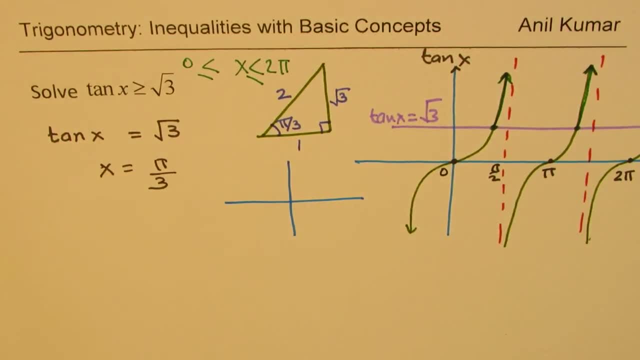 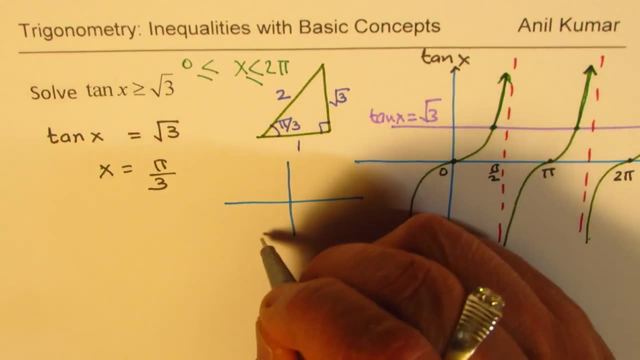 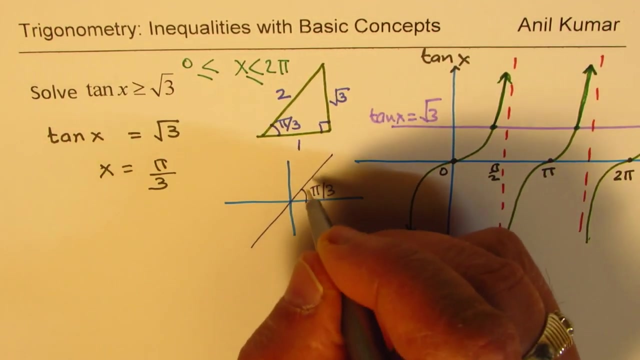 is to know when is tan positive and when is tan negative. Well, in quadrant 1 and 3, tan is positive, right? So pi by 3,. I could draw a line like this, indicating that this angle here is pi by 3.. And so this is 1 pi by 3,, 2 pi by 3,, 3 pi by 3.. This is 4 pi by 3. 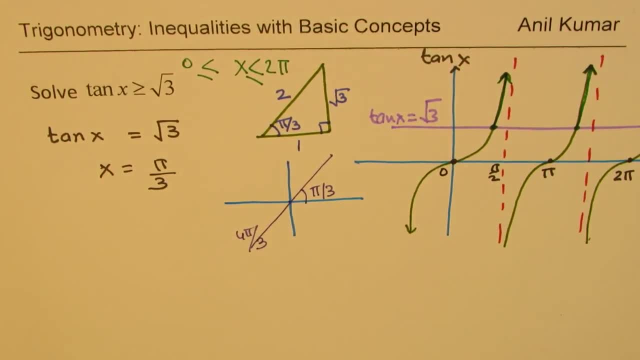 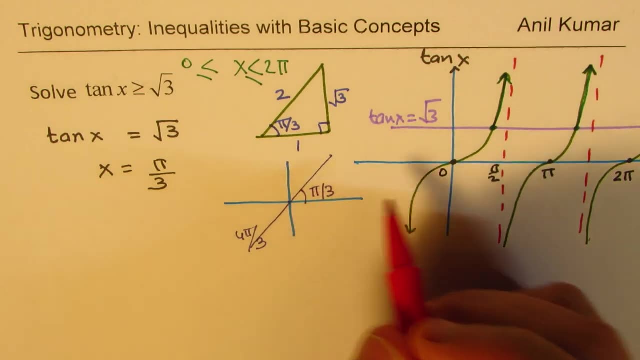 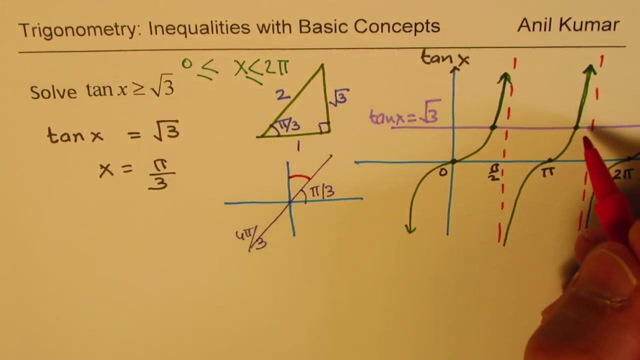 for us, right. So when we are saying that tan x is greater than, that means our solution lies in the interval between pi by 3 and 90, right there, correct. And also this portion which is right there. 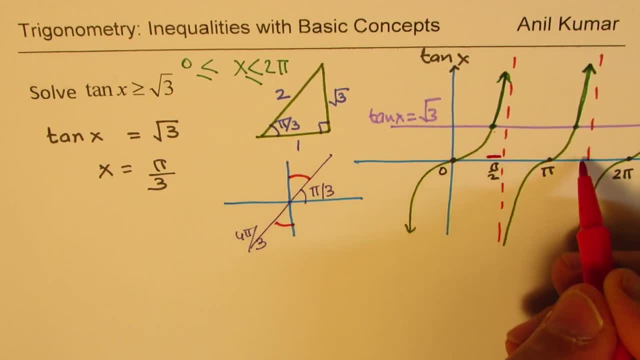 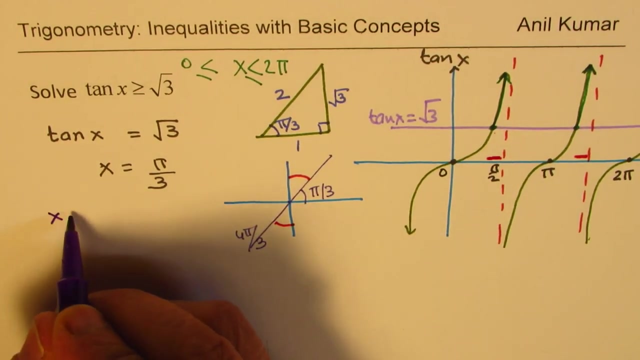 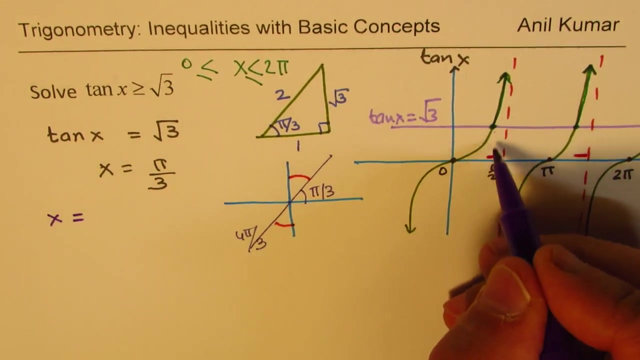 The interval is: is this? Do you see that part? That little bit of interval, is the one where our solution lies. So we could write the solution as the value of x will be equal to Now. it is greater than equal to right, So this point will be included. However, 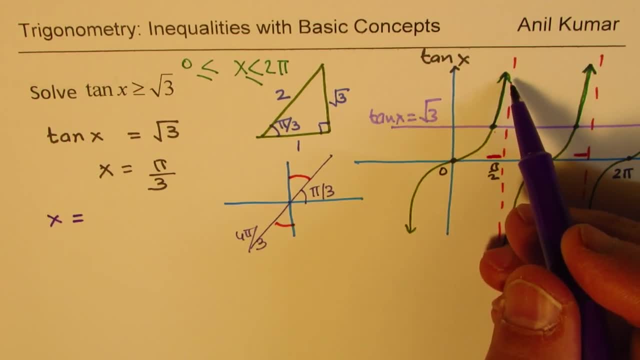 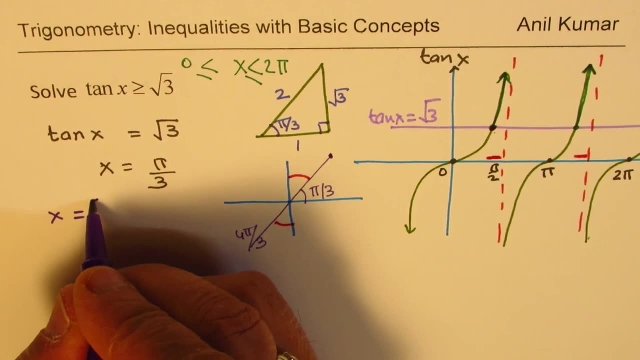 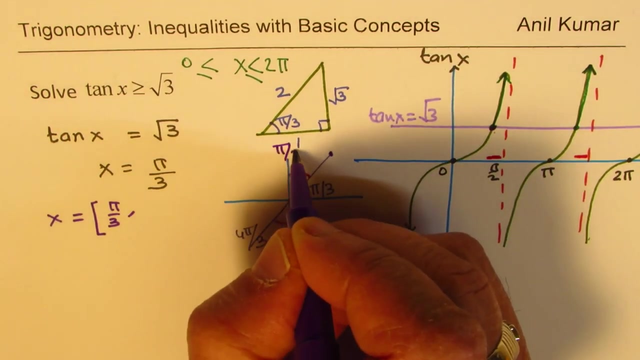 pi by 2 cannot be included since it is not defined at that point, Correct. So therefore this point here, which is pi by 3, right, will be included, So we can write this as from pi by 3 to pi by 2.. This is pi by 2, correct, 2 pi by 2.. However, 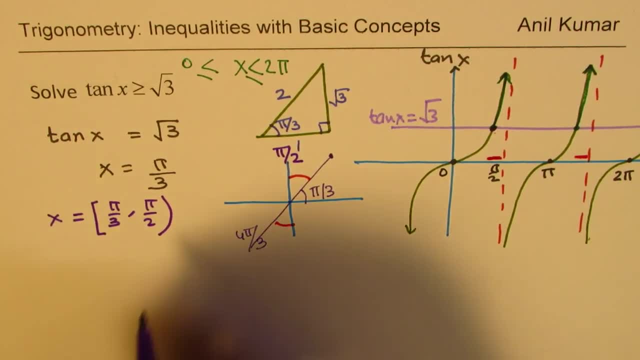 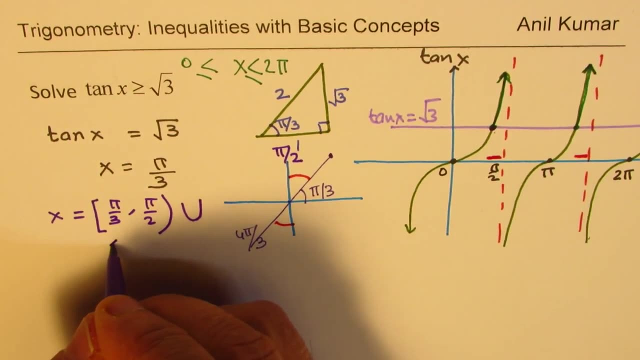 pi by 2 is not included. You get an idea, So that becomes the solution. Union means and this portion also right, which is from 4 pi by 3. Again, you should include 4 pi by 3.. 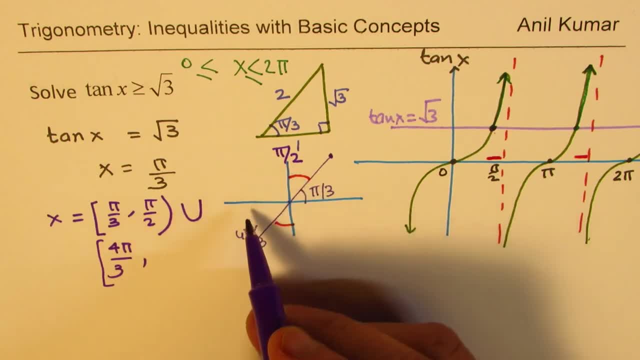 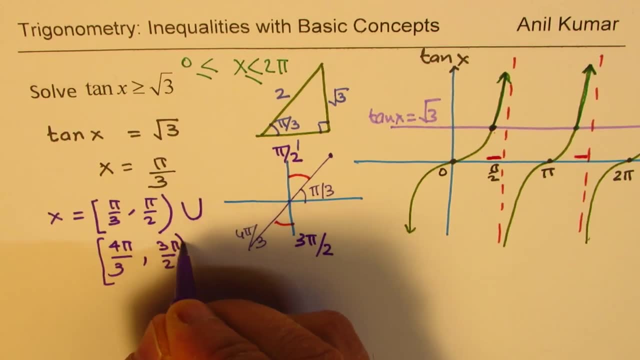 But you cannot include. this is pi by 2, 2, pi by 2, 3, pi by 2, right, So this is 3, pi by 2.. Does make sense to you? You cannot include this, So that becomes the solution for our. 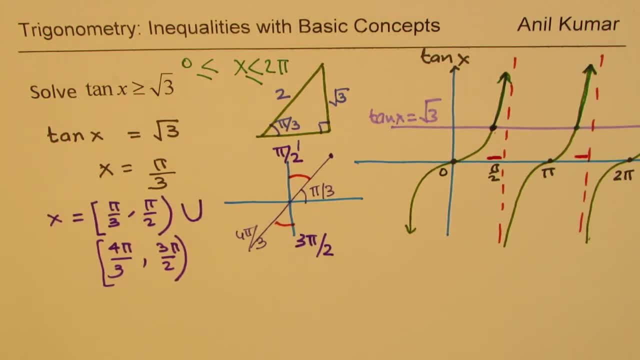 trigonometric inequality. Does it make sense to you? So that is how we are going to solve all these questions. So we will try to sketch a graph. We will try to relate the value from our special triangles: See the solution. 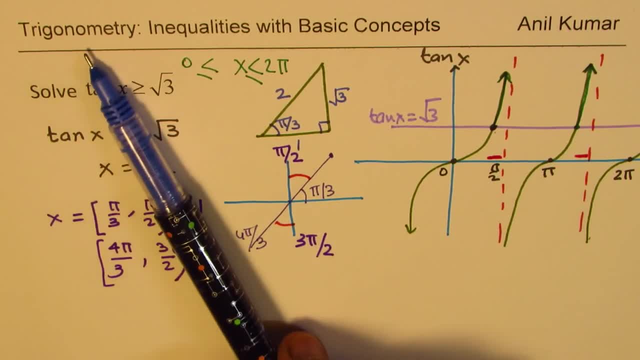 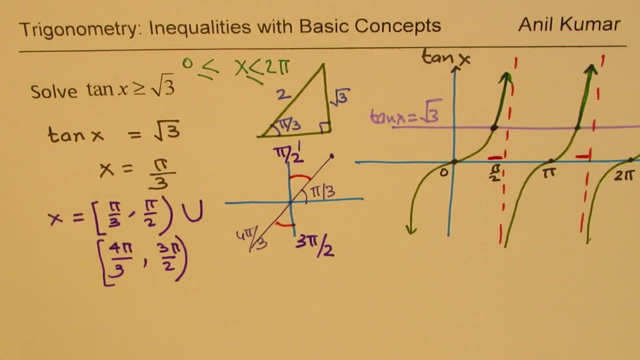 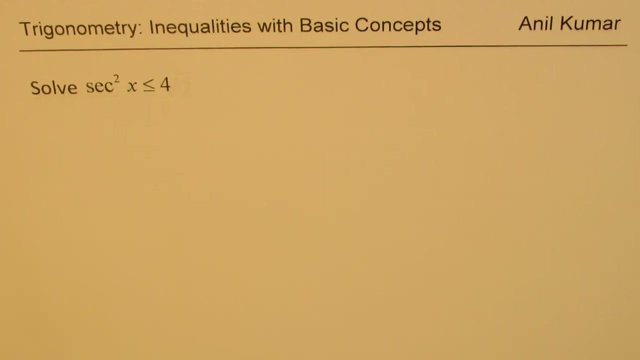 Write it down right Now. I have a list of videos working with trigonometric inequalities. I will provide you with a link on that, and there you can see other methods to solve trigonometric inequalities. Perfect, Let us move on and take the next question Now. this time we 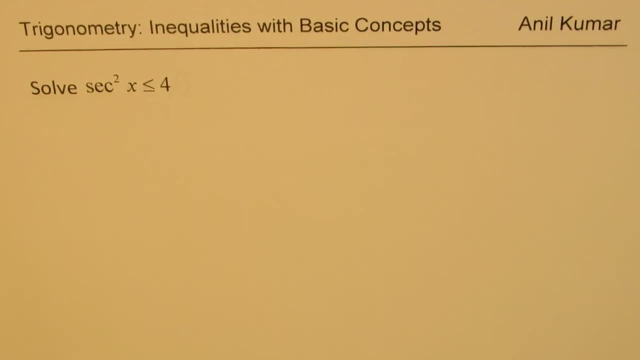 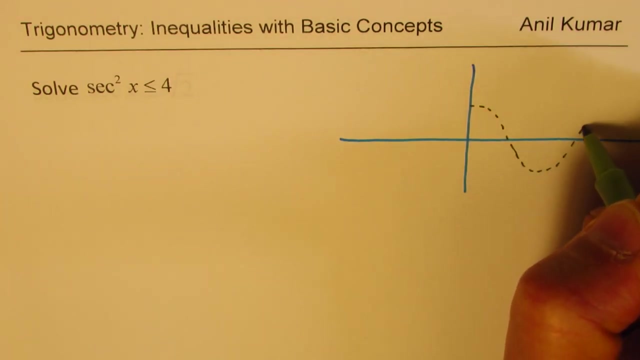 have secant square x less than equal to 4.. Now again, let us try to sketch the function. Now we are working, as I said, between 0 to 2 pi. So secant is inverse of reciprocal, of, I should say, of sine. 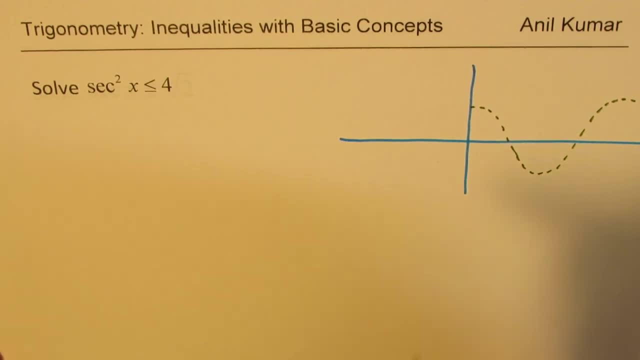 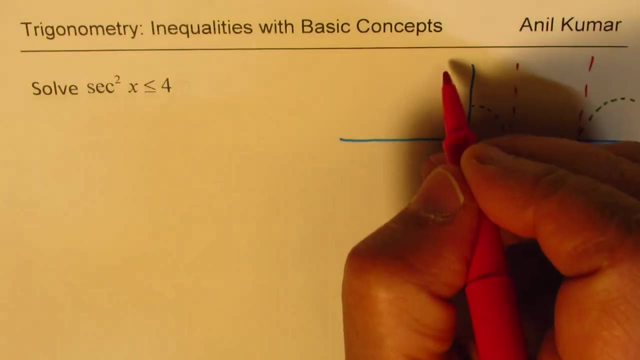 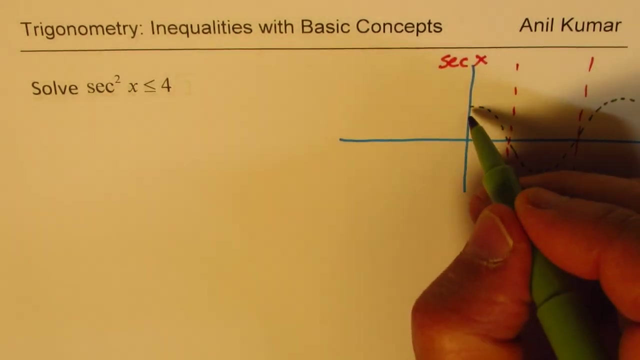 cosine function- right? So that is the cosine function graph which I have drawn at 0. there will be vertical asymptotes, right? So from here we will sketch secant x. ok, So let us first sketch secant x. ok, Let me just draw this, perfect, ok. Now, when we say secant x, 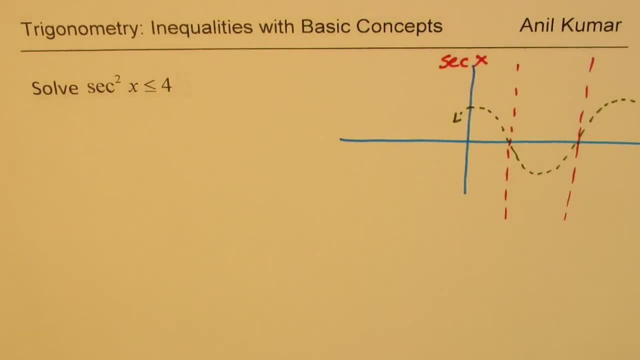 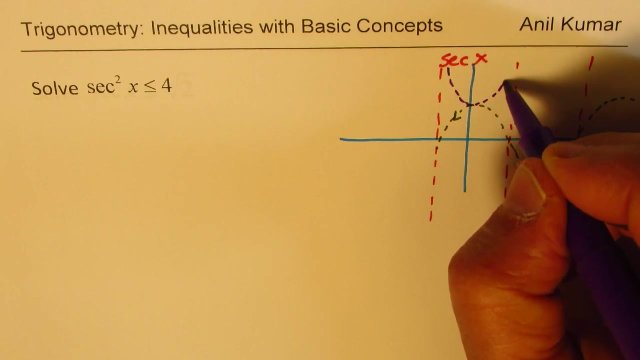 then, ok, let us complete this side also. it makes sense, right, because at 0 we have a vertical asymptote. that is the whole idea. So the value of this secant x will be kind of like this, right? Ok, Ok, Ok. 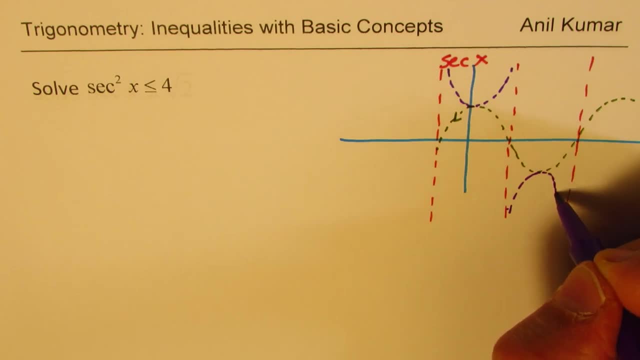 So on this side it will be kind of like this: So these dotted lines are not of our interest, they give a secant X, But we really are interested in secant square X, Right? So for secant square X, everything is positive, right. 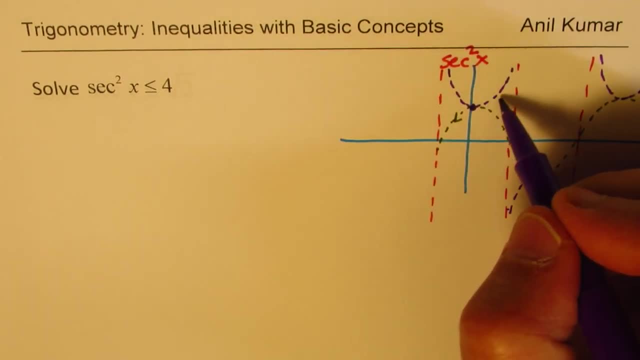 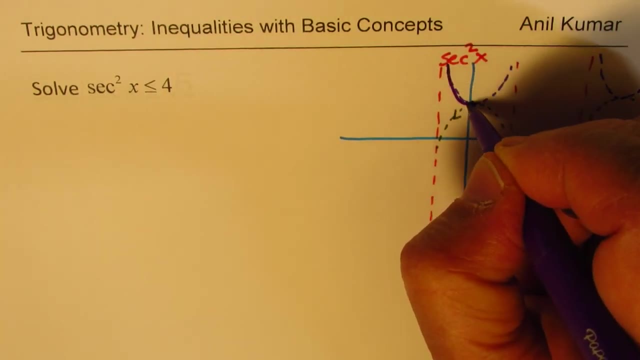 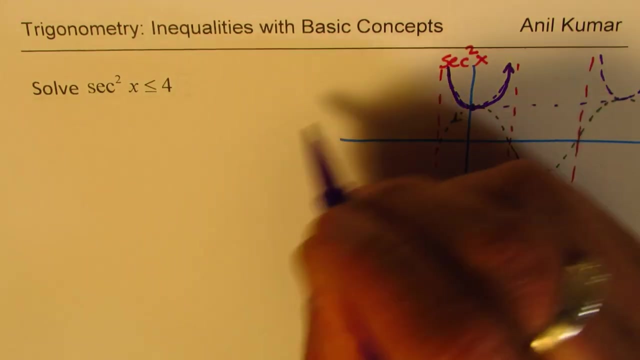 One remains one, one remains one. If it is, you know, a smaller value, it will be like flatter. So the graph will be kind of like this. Let's say, let me just Approximately- and here the minimum value is going to be positive- one for secant square X, right? 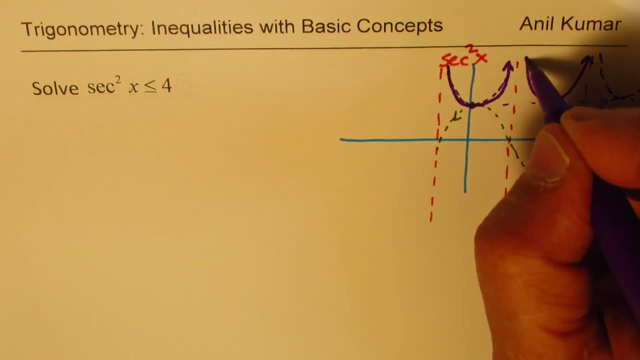 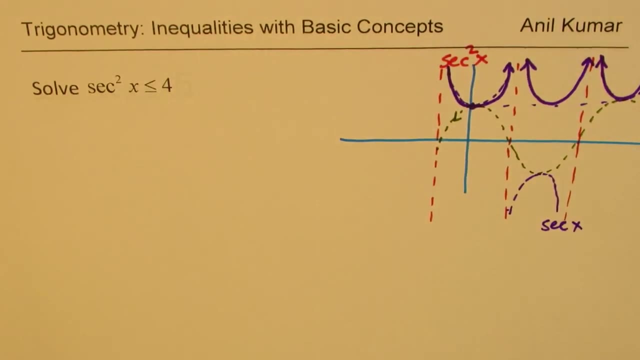 So we kind of get our value of the graph like. this does make sense to you, So I hope you understand the concept. So we have got secant square X now. Perfect, So secant square X is less than equal to 4. That means we will try to figure out. when is it 4, right? 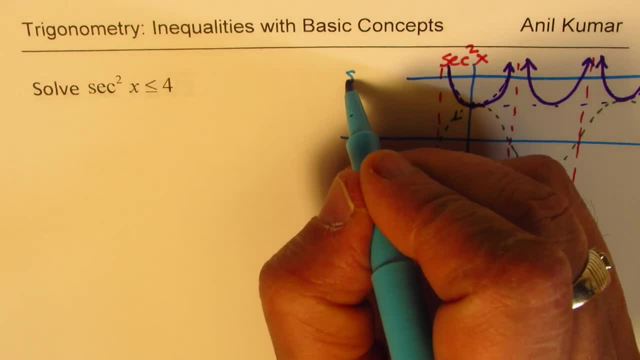 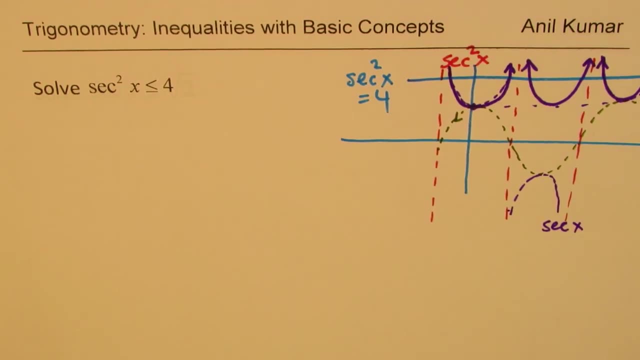 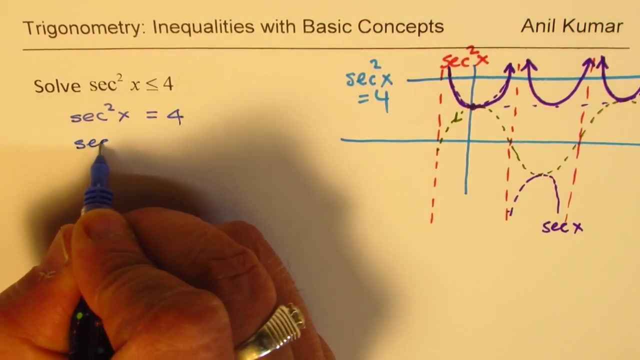 So so this is the point where it is 4. so we can say secant square X equals to 4 at this line. Let's find that value Okay. so we say that Secant square X is equal to 4. that means secant X is equal to plus minus square root of 4. 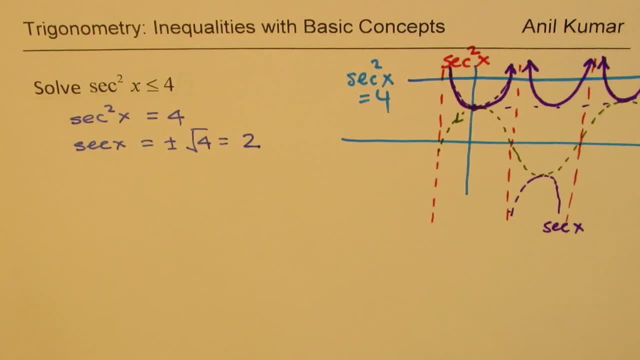 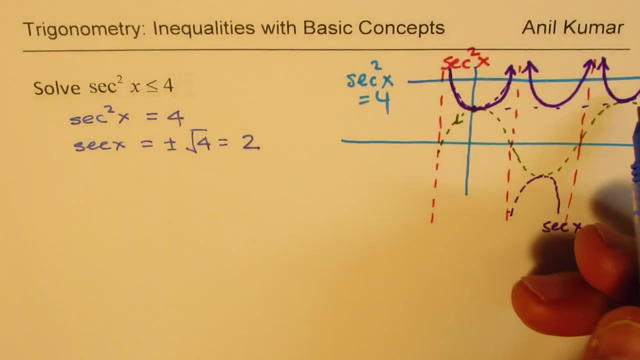 Which is, which is 2, right? So when is secant X Plus minus 2, right? so so What we are seeing here, secant square- is always positive, So we want it to be great. less than, I'm sorry, less than this. So we are looking for something below this. 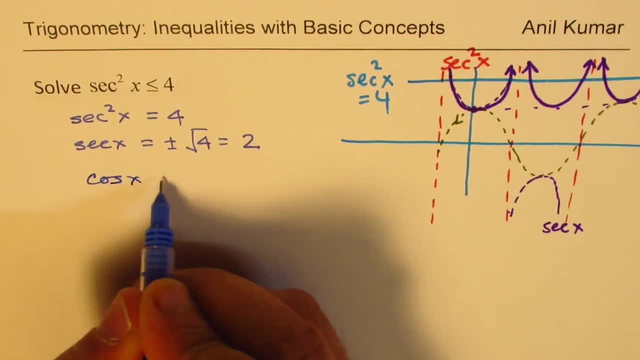 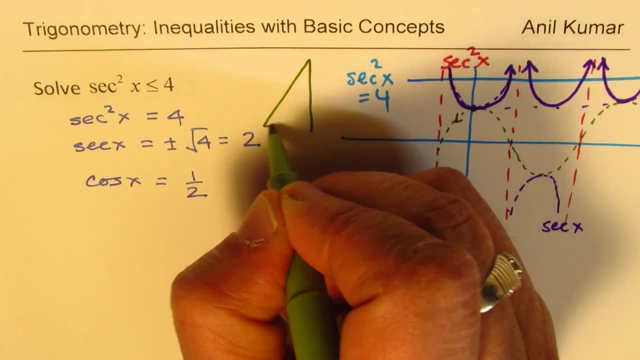 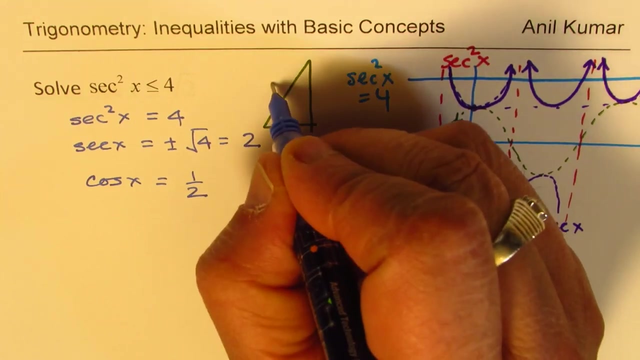 Okay, so we could talk about cos X equals to half. now when is cos X half? So again, get back to your special triangle, right? half means you have to look into again. add up This side right, so which is pi by three. So cos X is half means X equals to pi by three. 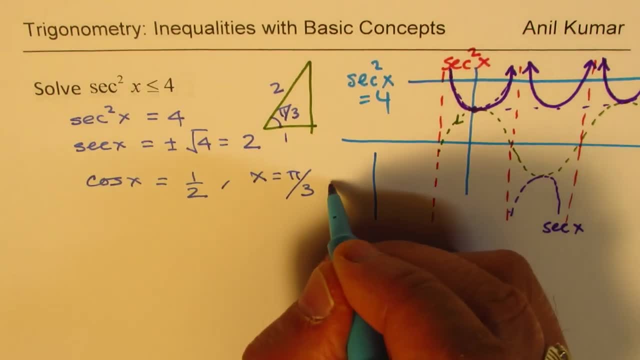 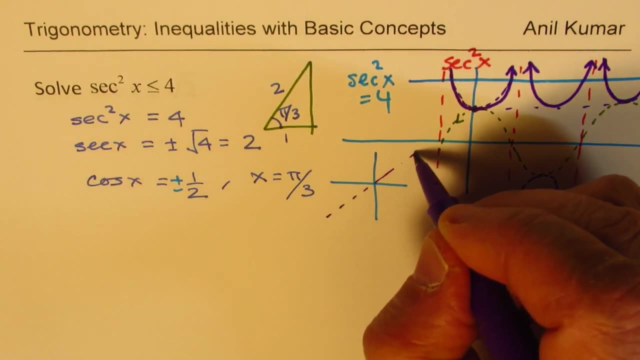 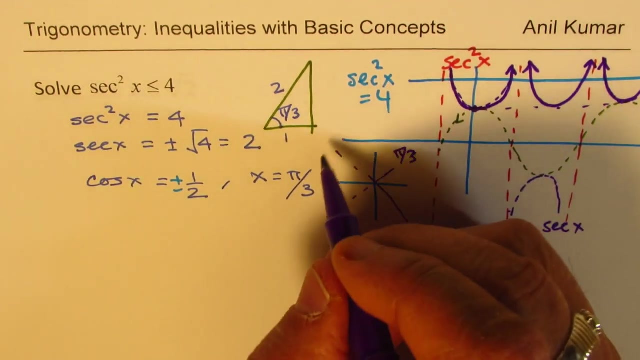 How many times in this particular graph? now we are looking for both plus and minus, right, We are looking for both plus and minus. so that means, Okay, now, this is not really pi by 3, but you know. So what we are trying to say here is: this is pi by 3, then we have to pi by 3. 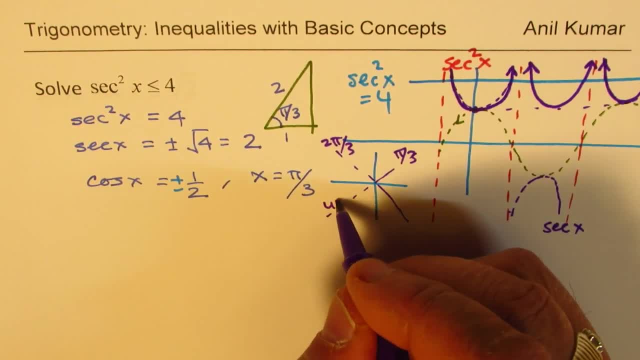 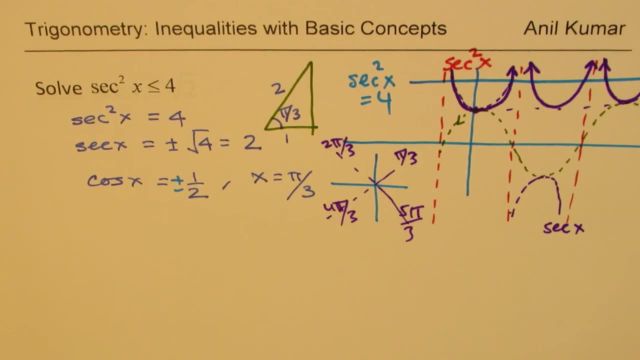 this is 3 pi by 3. so this is 4 pi by 3, right, and this is 5 pi by 3. so these are all the critical numbers which we have to look into right now. when is secant square X less than 2? that means secant X is between 2 and minus 2. you can say: 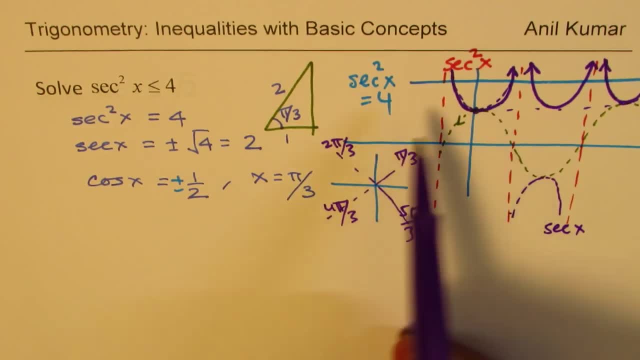 less than 2, right, so secant square X is this and this. what we are looking into is cos X is between plus minus half. that is what. if you're looking into is it okay? so if you look into the cos function, cos X is less than I mean less. 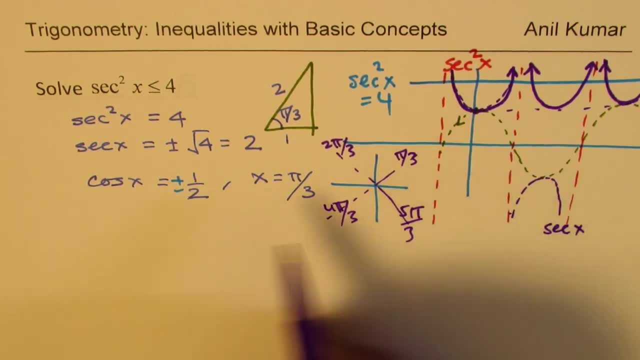 than equal to half. so let's look into the cosine function. so at half is that pi by two. three, right, pi by three. so let me drop a line here using a different ink. that'll make sense, right? so let's say this is one, so this is my. 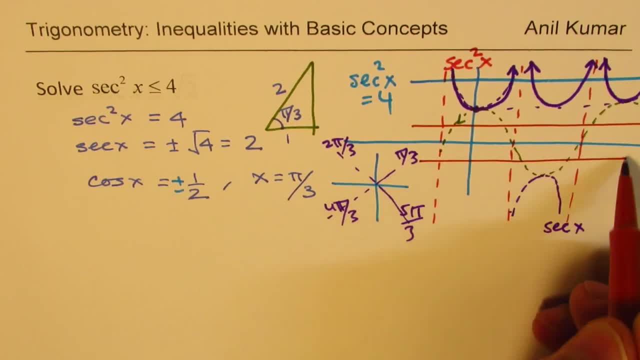 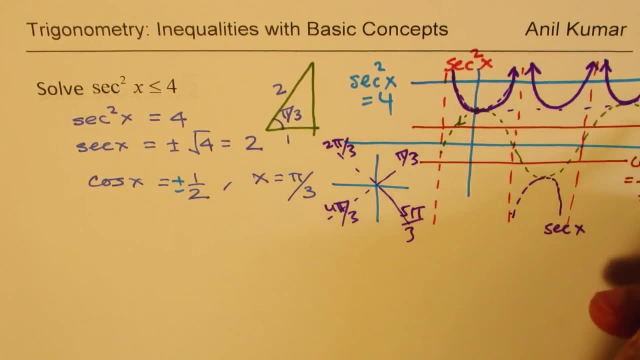 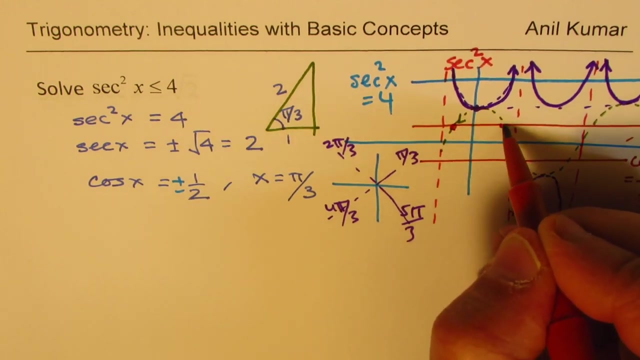 line for cos x being half. So this is cos x equals to minus half, and this is plus half for cos x, right? So that is for cos x. So those are the points of our interest. Those are the points of our interest. Do you get the idea right? So even these points right. These are the points. 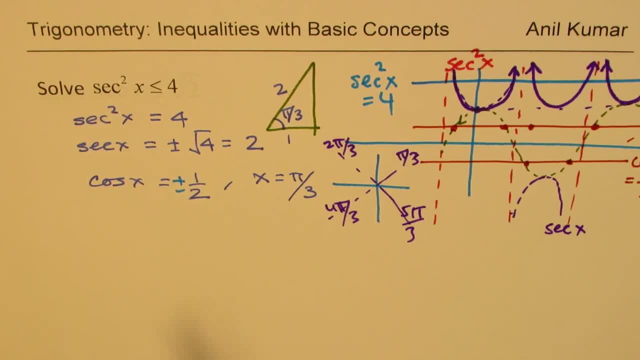 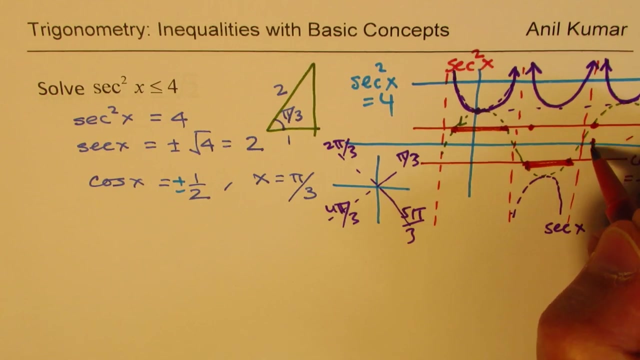 of our interest, correct? We want the value of secant x to be less than something, right? So less will be, as you can see from the graph, in between these points, correct? So in between these points is what we are looking for. Got it Now? our domain is only up to this point, right. 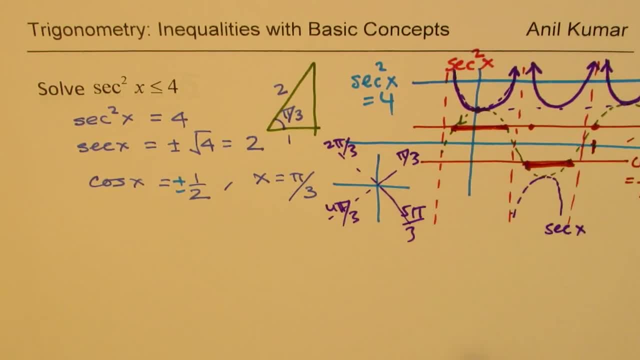 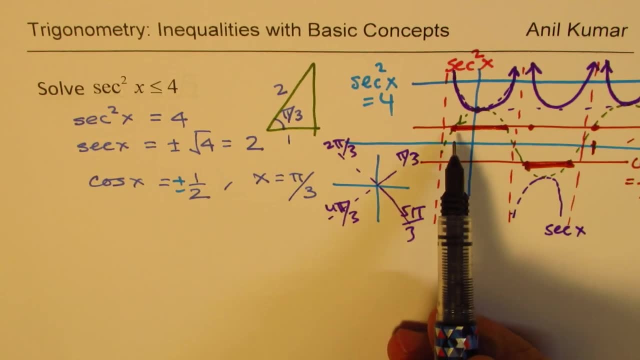 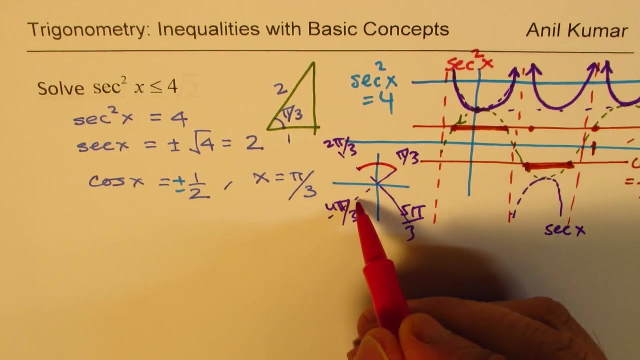 So only up to this point. So these are the two intervals which give you the solution. does it make sense to you? perfect, okay, so now we get our solution, that is to say that we are looking for something which is in between this and which is in between this. those are the points. 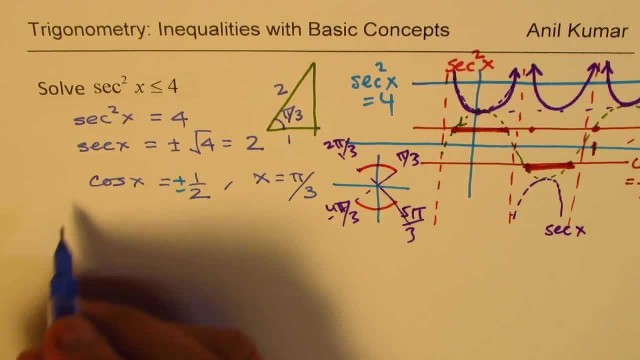 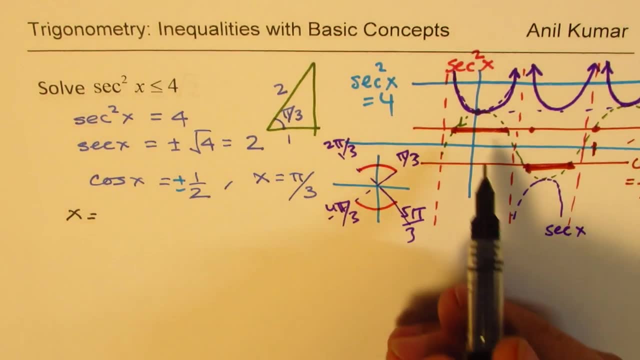 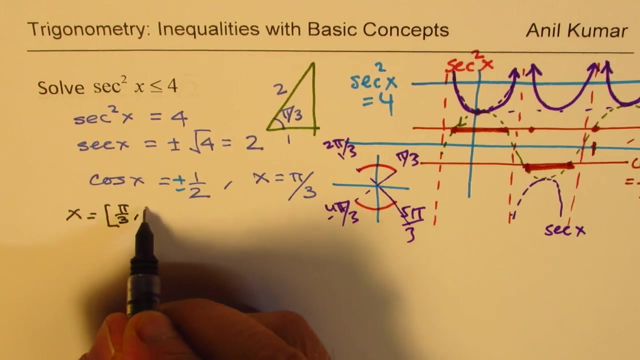 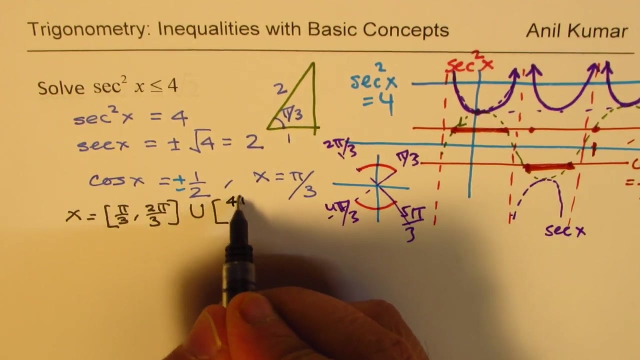 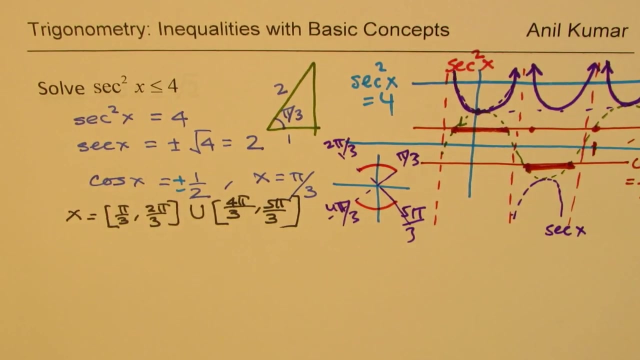 marked there, so we can say that the value of x is equal to now. both are included. right, there are no restrictions on this. so it is included between pi by three to two pi by three, and also between four pi by three and five pi by three. does it make sense? so, in these two examples actually, we 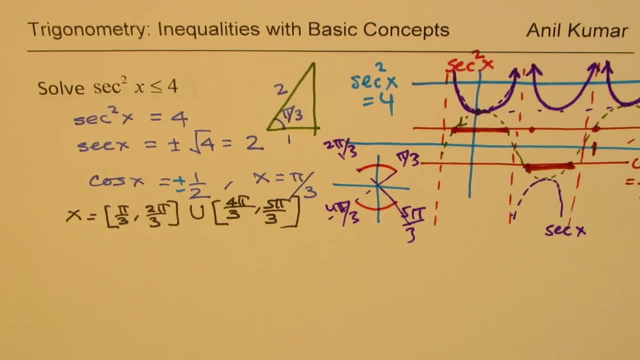 have covered the whole variety. we have looked into a trigonometric function, the primary trigonometry ratio. you also looked into the secondary trigonometric ratio, the reciprocal and also the square of that. so i hope with this you should be in a position to answer the rest of the equations right. so 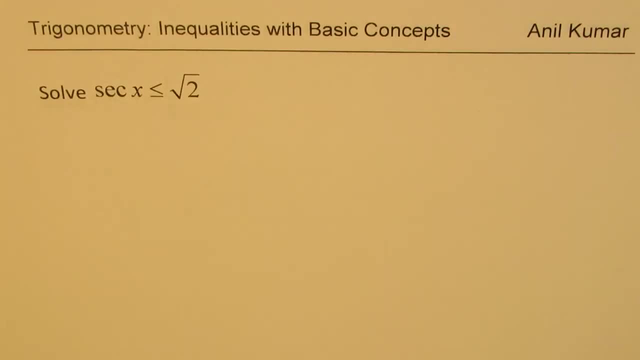 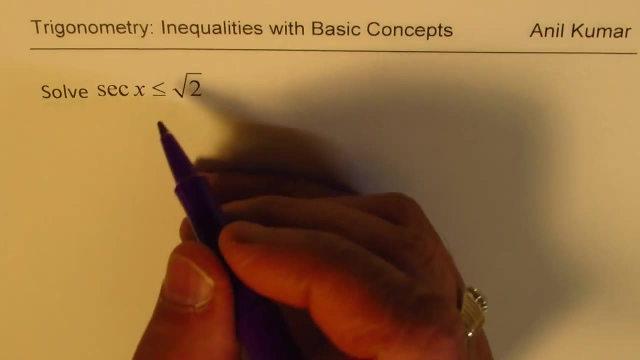 let's share the next one. we are not talking about secant x less than square root of 2, so how will you do this? well, when you get this secant x less than square root of 2, you can also write this as 1 over cos x. 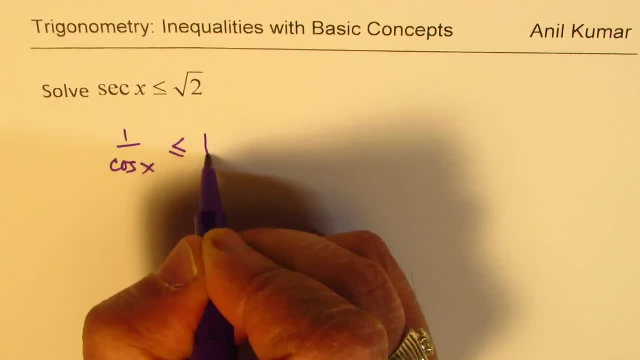 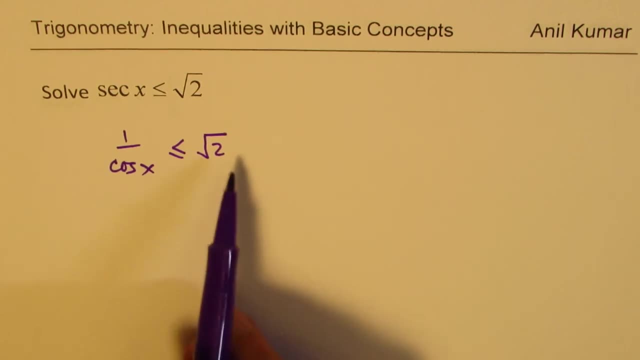 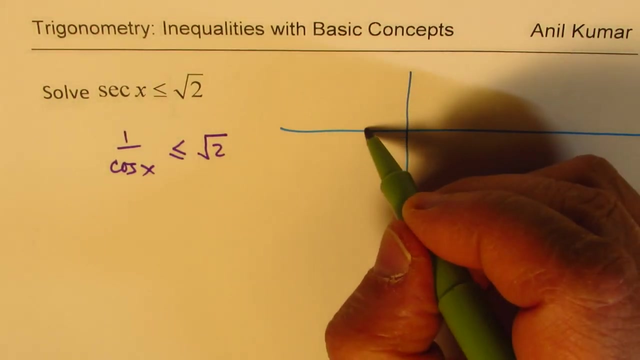 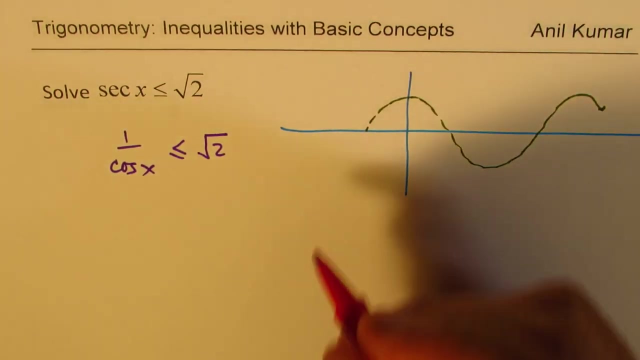 as less than square root of 2. right, that is what it is okay. now what you have to look into here is: we'll again sketch the graph cos x function. secant x is reciprocal of cos x, so you can write this as 1 over cos x, less than square root of 2. 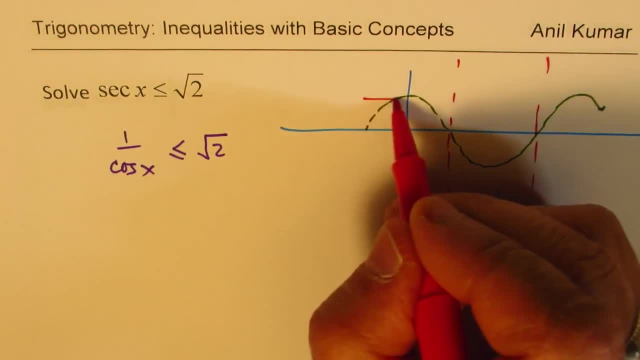 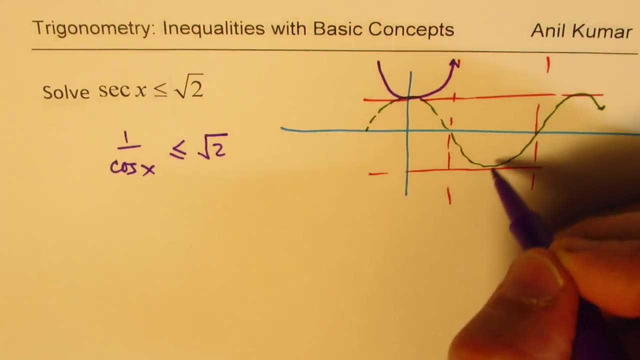 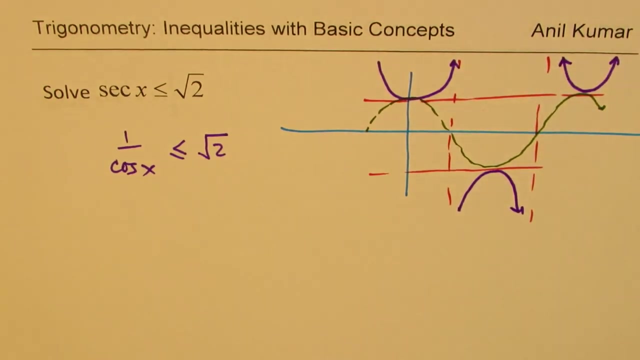 so there are vertical asymptotes, right. the graph will be kind of like this, as we did last time, but this is not squared, so you'll have negative and positive, both. right, you want secant x to be less than half. so what are you looking for? you are looking for something which says: 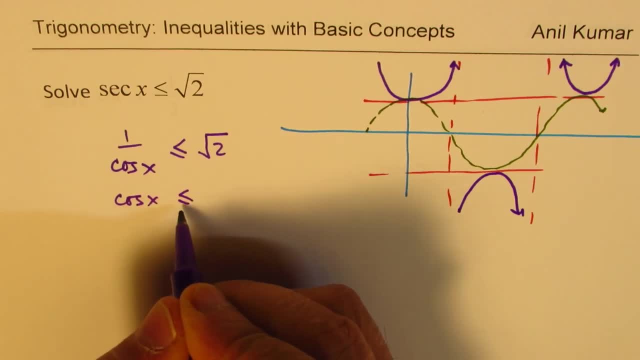 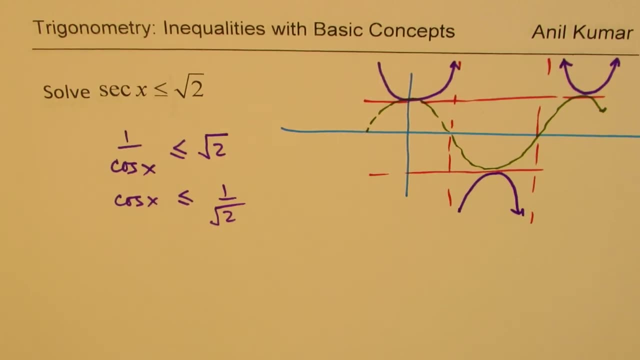 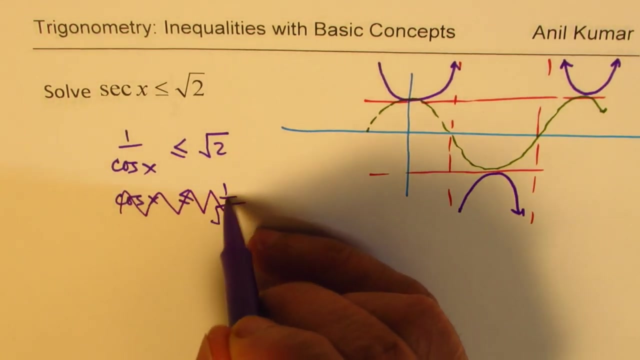 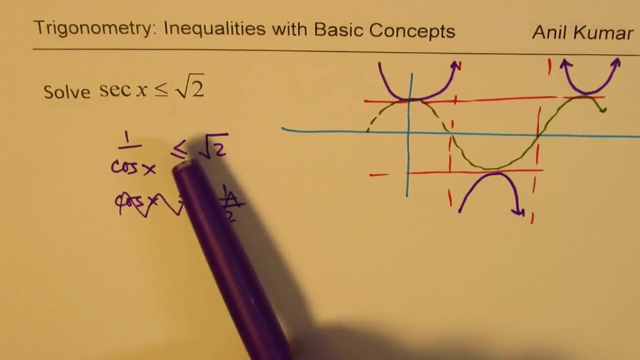 which is square root of 2 special. when you separate, scrik off every good step. this is incorrect reverse contract. let's try to do with the what, this particular function itself. so what we will see in in the first phase is fine. this is a littleБ. 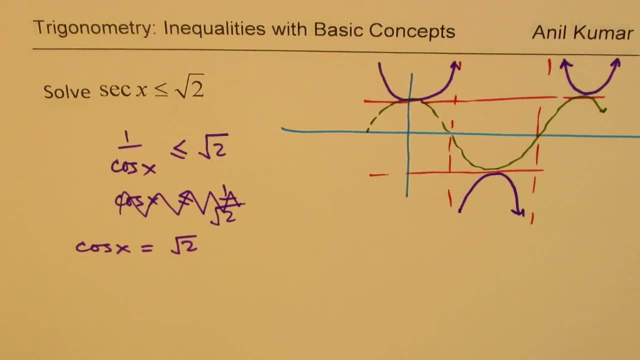 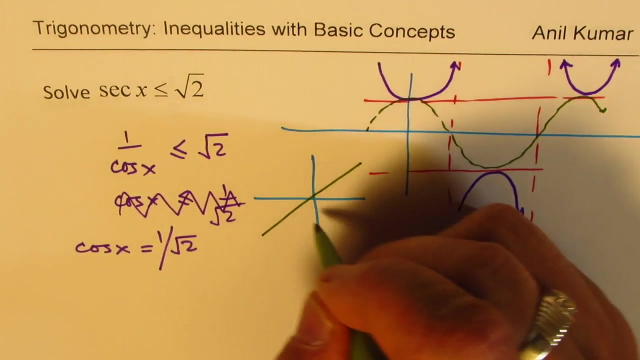 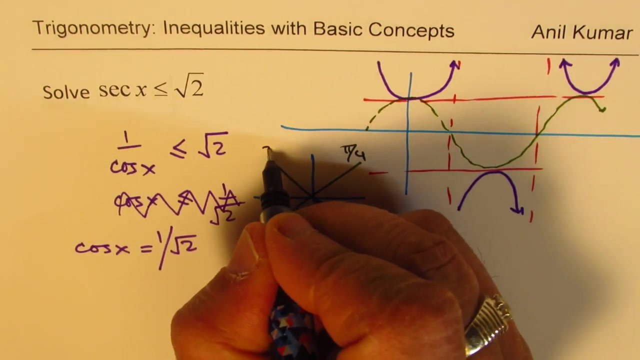 to square root of 2. that is also a part of our solution. right 1 over 2. I'm sorry, when is cos X equal to 1 over 2? now, if you look into again your coordinate plane, cos X is 1 over square root 2 for the values. when it is pi by 4, right 3 pi. 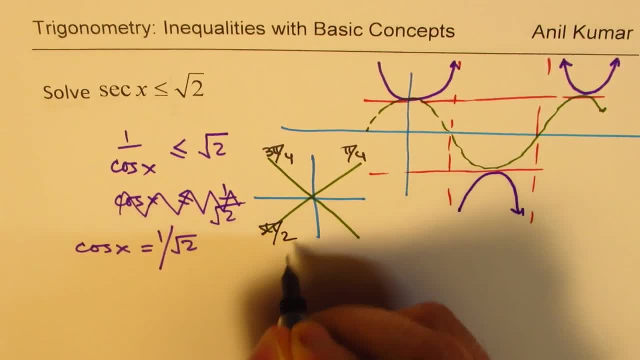 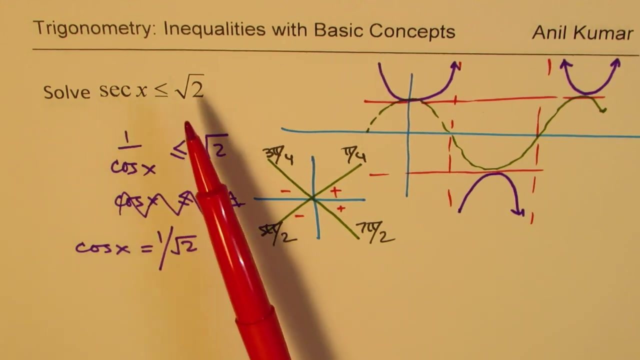 by 4, 5 pi by 4 or 7 pi by 4. now, cos X is positive in these coordinates, right, negative here. so we want a value which is less than this. so if it is negative it is always less than remember that part. so all this is included. negative is: 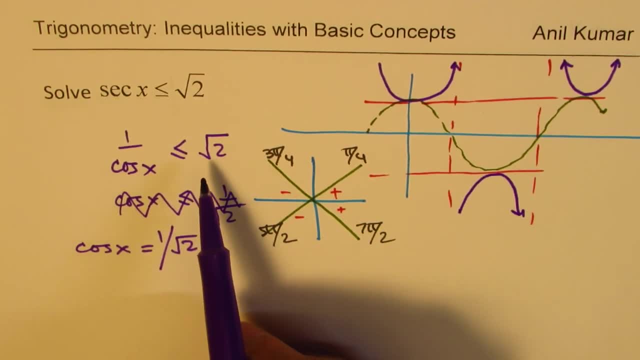 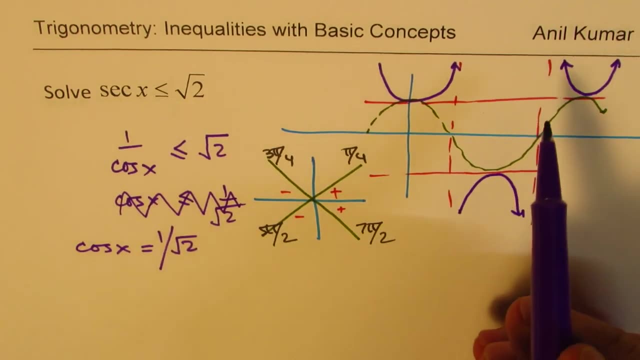 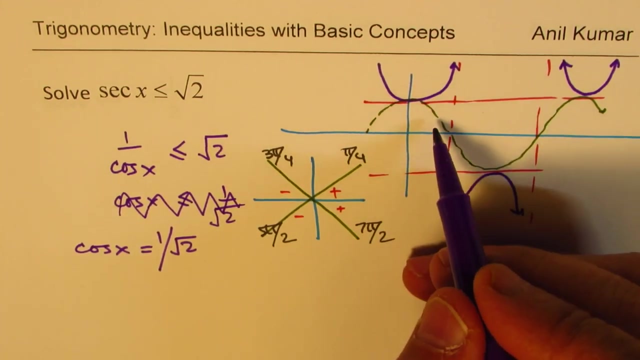 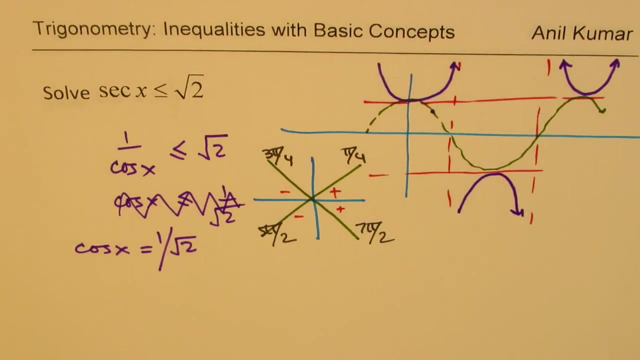 always less great. so when we are saying that we are looking for secant X right less than square root of 2. That means here: so 1 over square root 2 will be on the cos x, the 45 degrees right. So those are the points. So let's look into the cos x points of square. 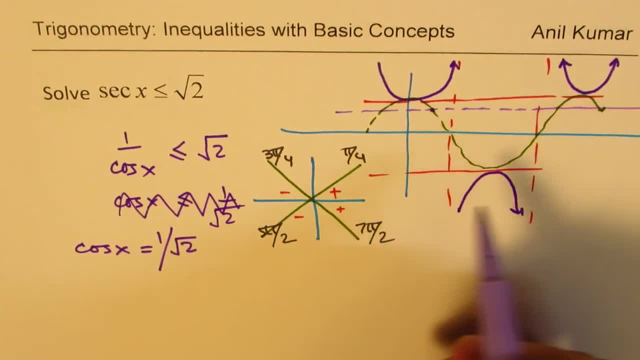 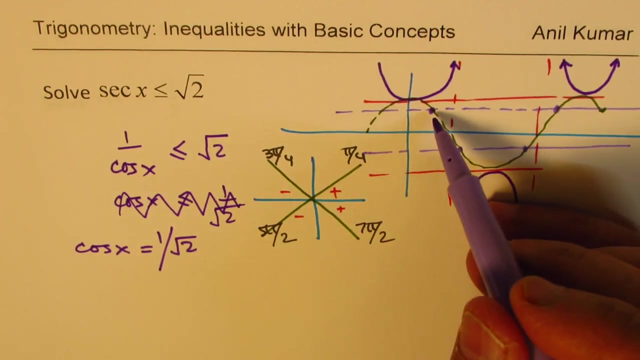 root 2 first, and also negative square root 2.. So we do get these points right Where it is square root 2 and those points are clearly marked here. where it is square root 2, right Now all these negative values are less than square root 2.. So definitely we have a result. 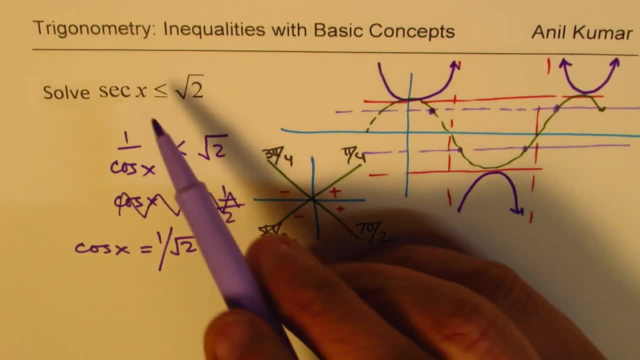 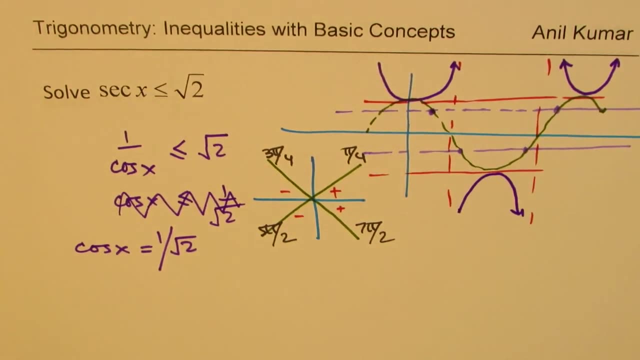 here, which is clear when it is within the domain Of secant x, but less than square root 2.. So 1 over square root 2, let me sketch that also in a different ink. This is nice. Now we haven't used this color, So let's say: 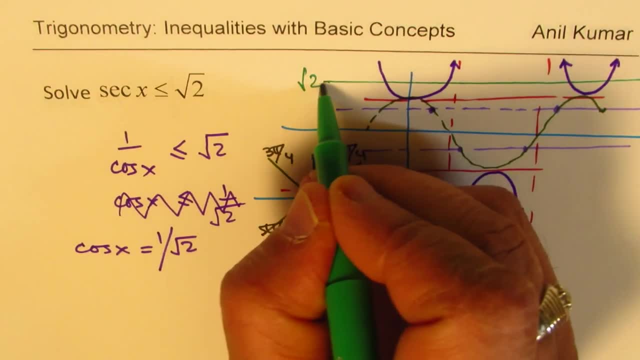 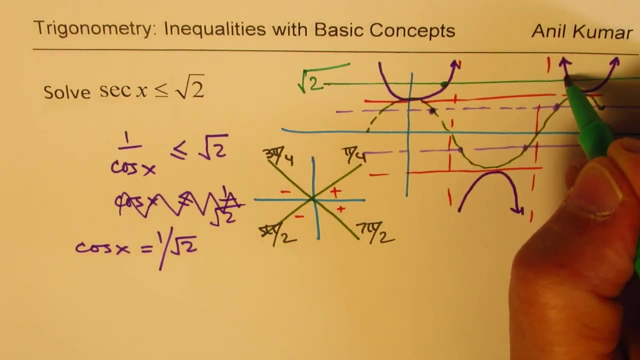 this is our square root. So we are looking for this graph. lower than that, right? So this corresponds to that value. You get an idea, right? So these two values which you are looking into, they We have to look into this value, right? Those are the critical points which we are looking. 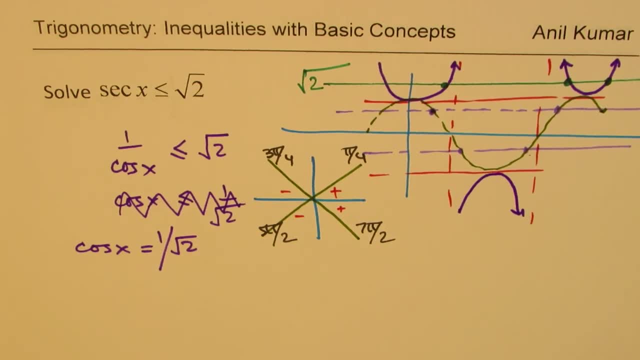 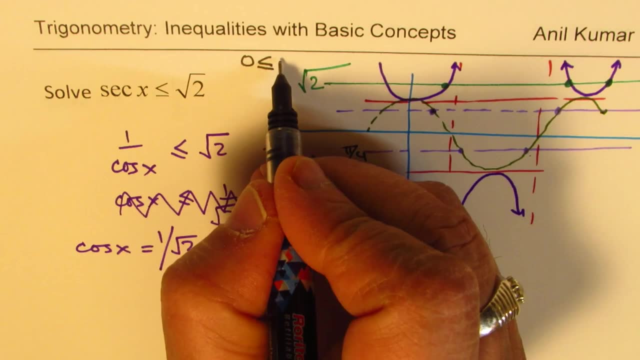 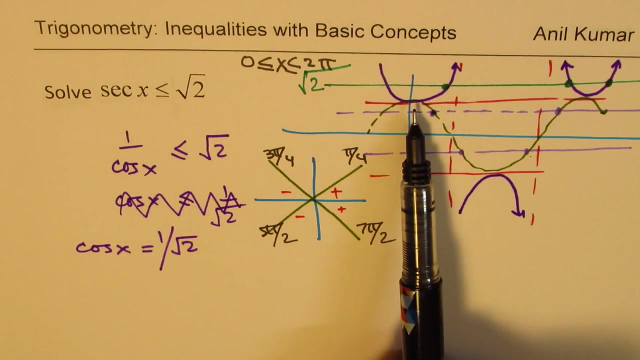 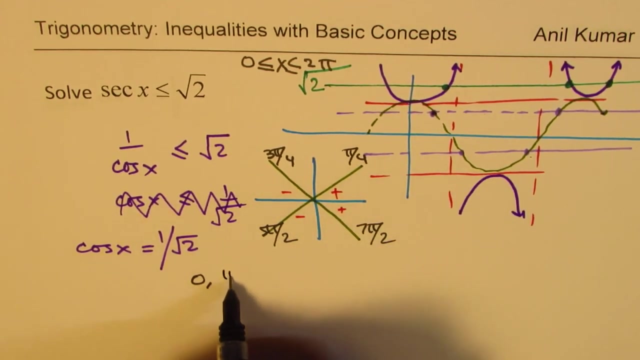 at Now. from here, what do you conclude? Between the interval 0 to 2 pi, the solution should be what? From 0, it goes up to this point without any problems, right? And then it increases. So the first interval is from 0 to pi by 4, correct. So in this interval it is less. 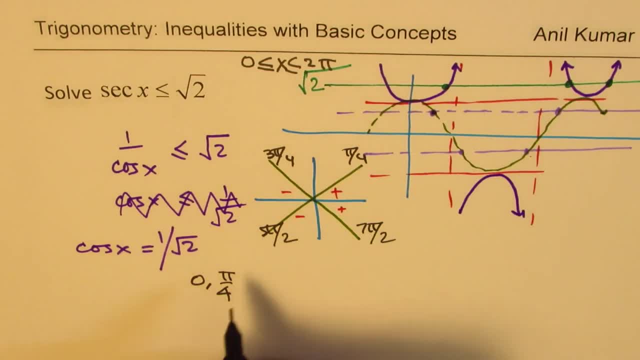 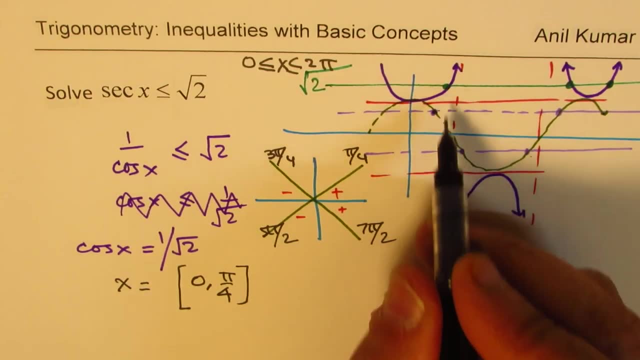 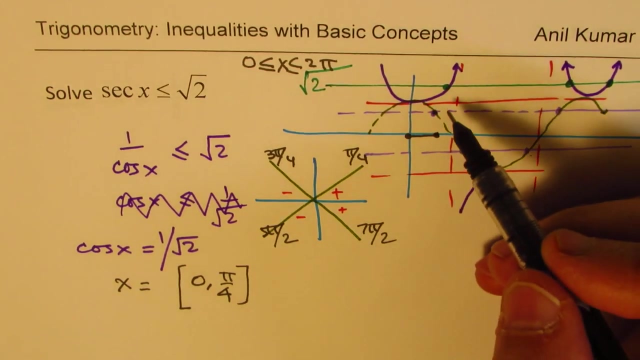 than square root 2, both included. After that it goes up. So that is the value of x. So between 0 to this, up to this point, So in our domain we get our answer from here to here, right? Then it goes up. 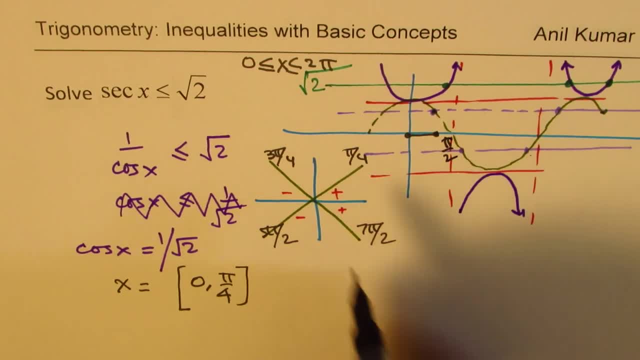 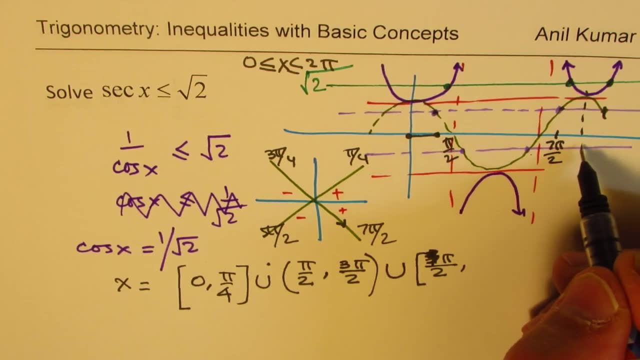 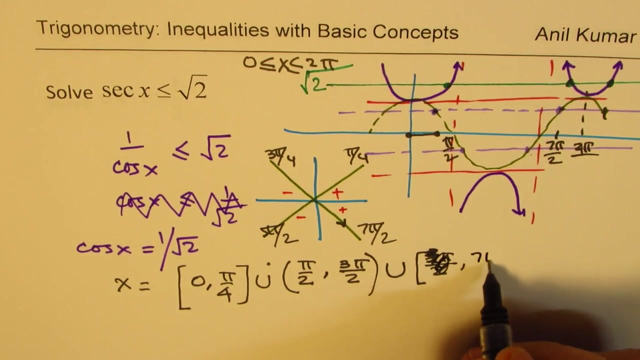 Then after pi by 2,, it is. We see here that from 7 pi by 2, to 2 pi, it is again below square root 2, right? So let me rewrite this: 7 pi by 2 to 2 pi. Is that clear? 2 pi will be included, correct. 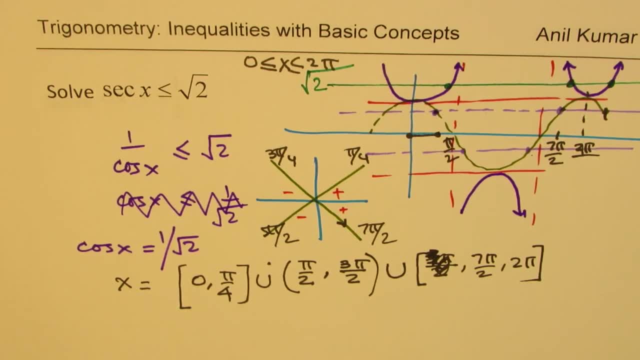 So that is how you get the domain for x. Is that clear to you? Perfect. So what you could do here is that you could analyze the graph and write down the answer quickly Using graph. it is much, much simpler Now. based on this, you can actually solve the rest of. 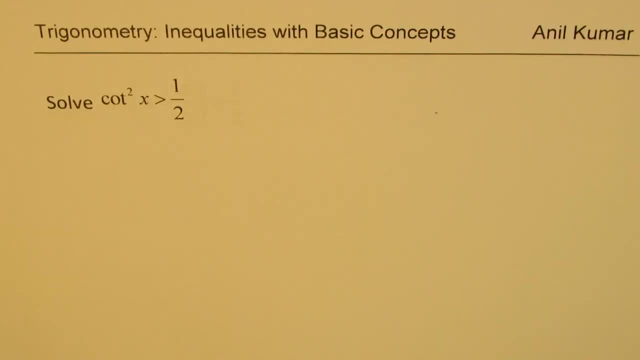 the questions. Perfect, So I'd like you to pause the video, answer the rest of the questions and then look into my suggestions. Correct Cod square x: greater than half. I'd like you to pause the video. Let's take a small break here and after the break we'll continue. 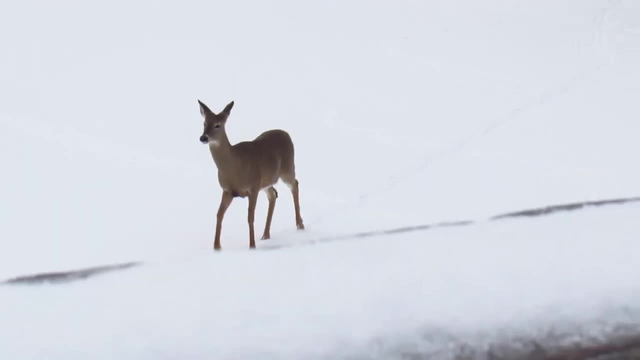 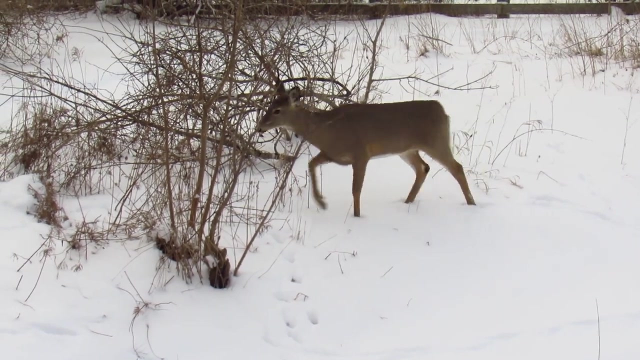 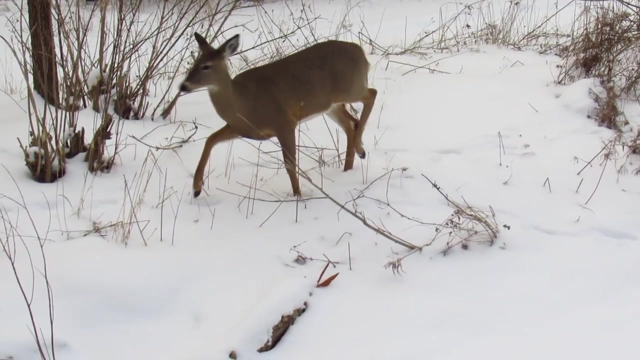 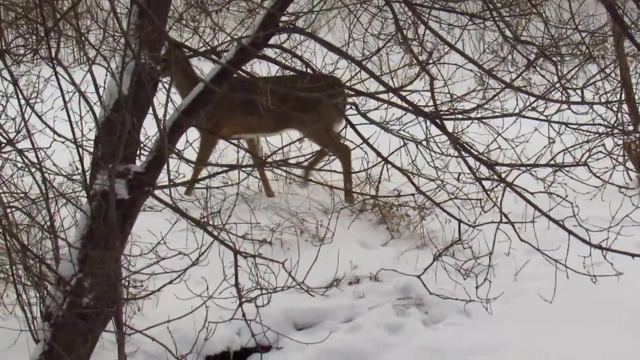 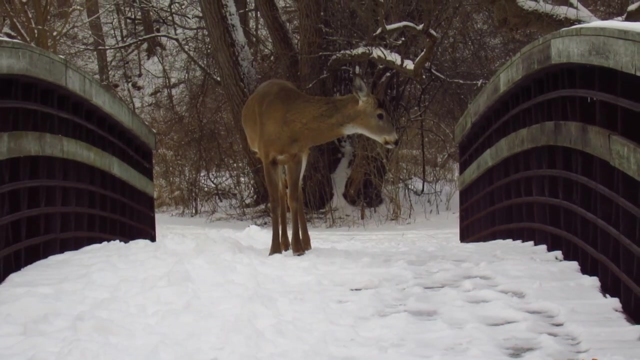 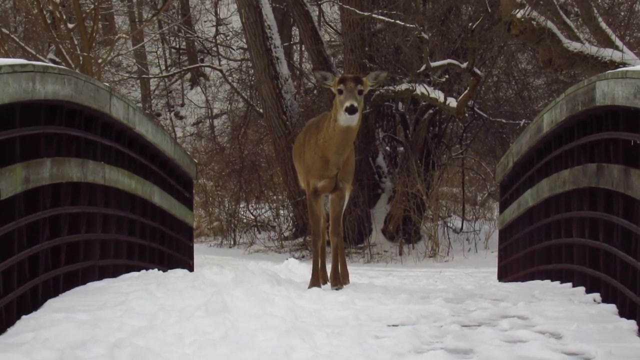 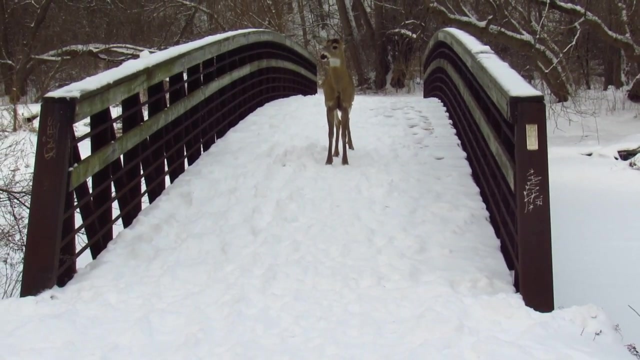 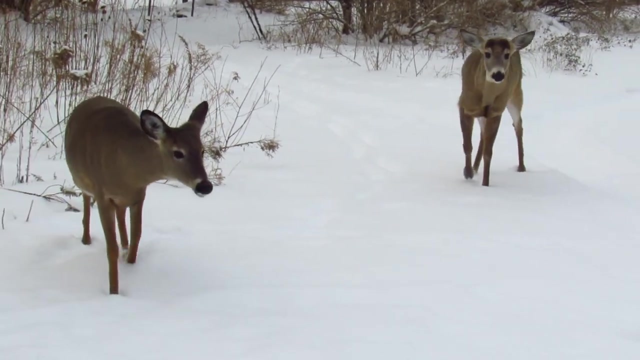 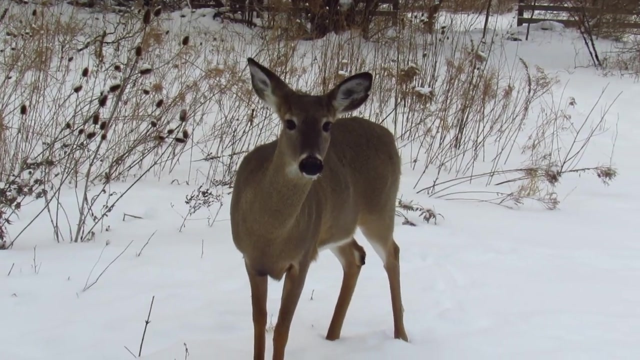 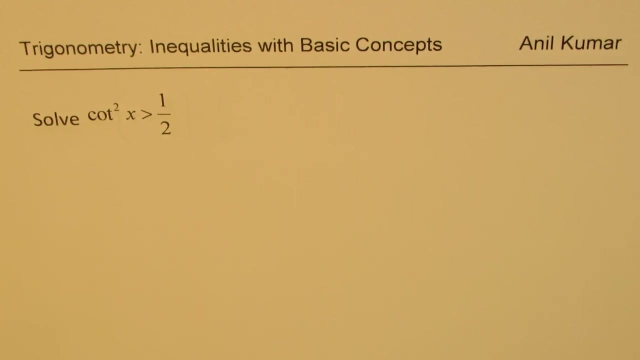 Cod square x: greater than half. Cod square x- greater than half. I hope you enjoyed the wilderness of this beautiful region. There's a lot of snow around, but still we see quite a few animals and birds. It is very refreshing. So, with a fresh 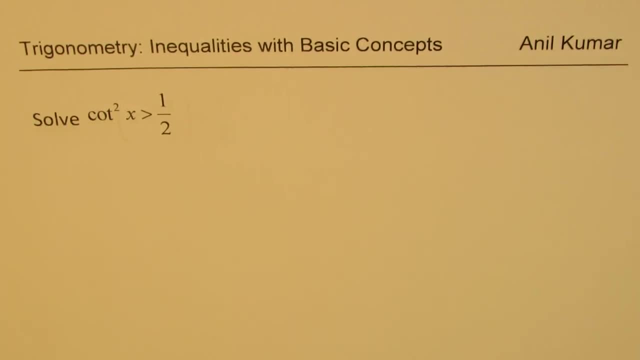 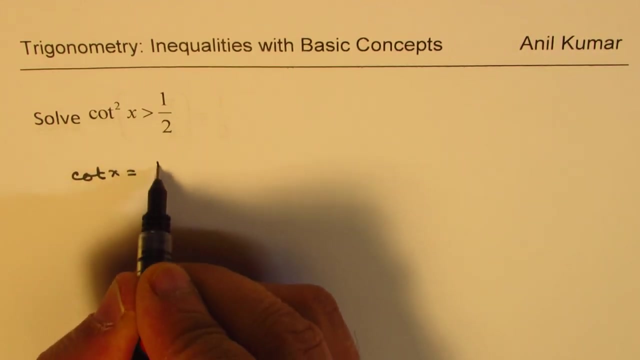 mind. now let us try to solve the remaining questions. We are working on the inequality cod square x greater than half, 1 over 2.. So that is to say, we need to now figure out what is cod x equals to Cod x? should. 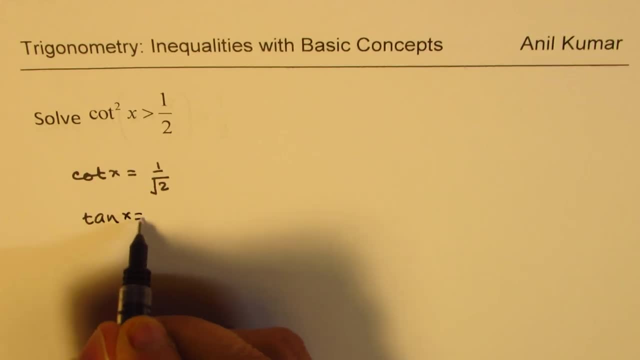 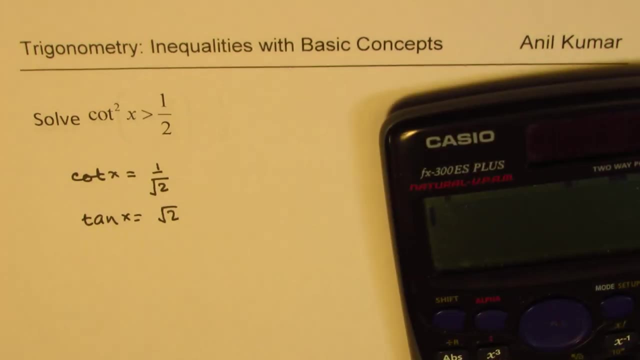 be 1 over square root 2, or tan x should be equal to square root of 2.. Now to find this value, we need to use calculator right. Remember we are working in the domain from 0 to 2 pi. 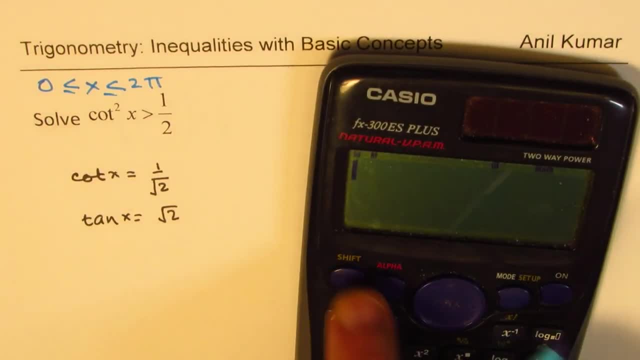 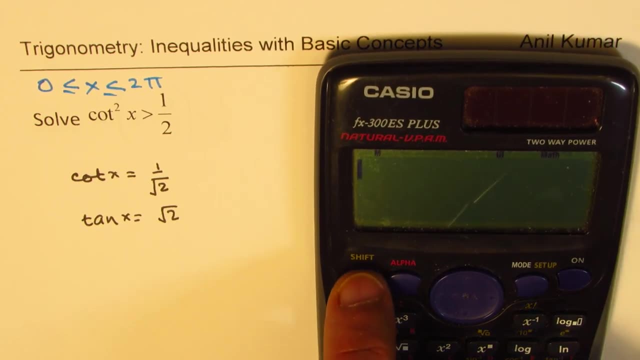 That means in radius. So let me first set The calculator in radians, right? So that is that option for radians, and we'll find when is tan x equals to square root 2. So we'll do square root tan, inverse of square. 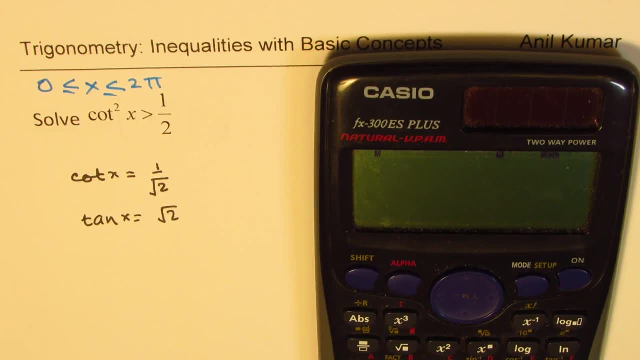 root 2, right. So what do we get? We get 0.955.. So we get x value of 0.955,- sorry, 55. Right, So if we are going to take our尺, then we're going to subtract 0.955.. We're going to subtract. 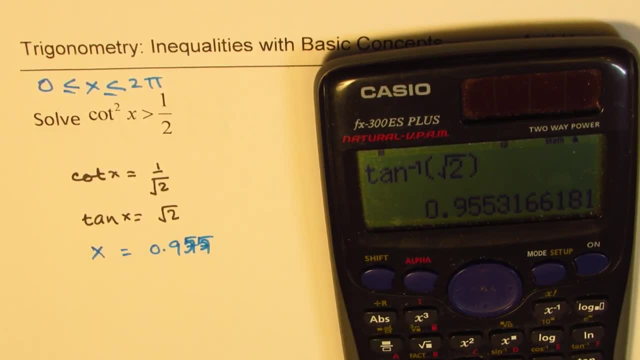 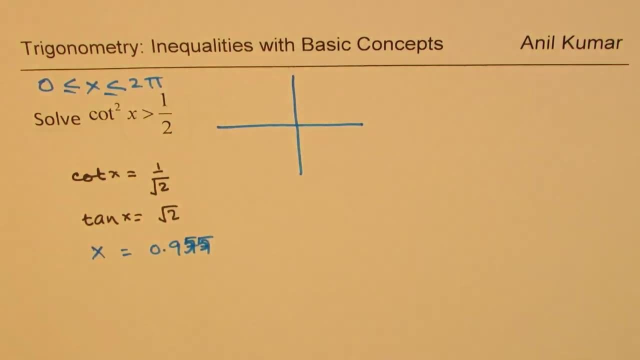 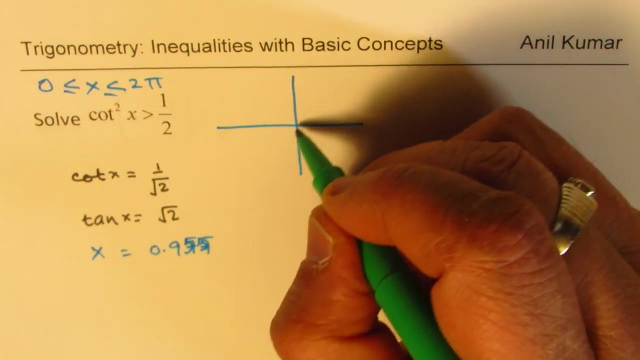 it. so we'll be getting 0.955.. Right, 0.955.. right, That is what we get, right. So what we know here is that we are actually looking for both. So, using calculator, I found the value for square root 2, right. So what we can find? 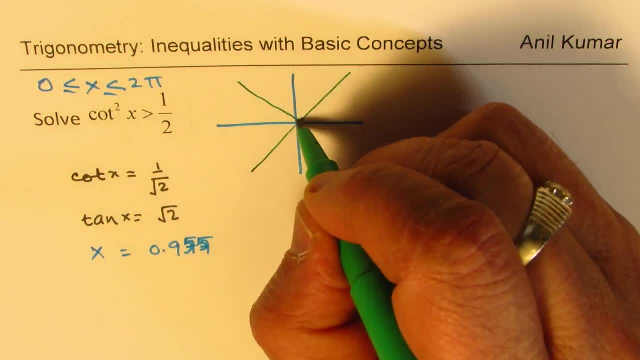 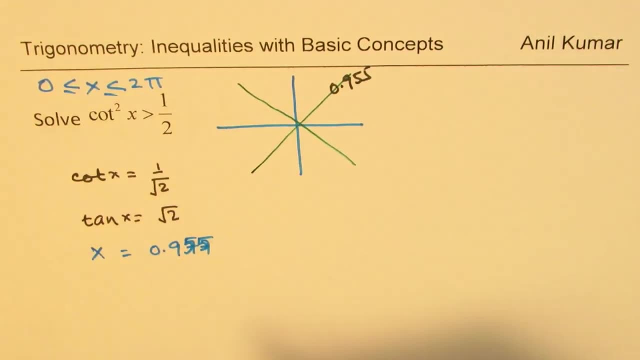 all of this. So let us say approximately, let us just draw our lines. We know this value here is 0.955, right? So the other value will be: we can add pi to it, right? So if I add, 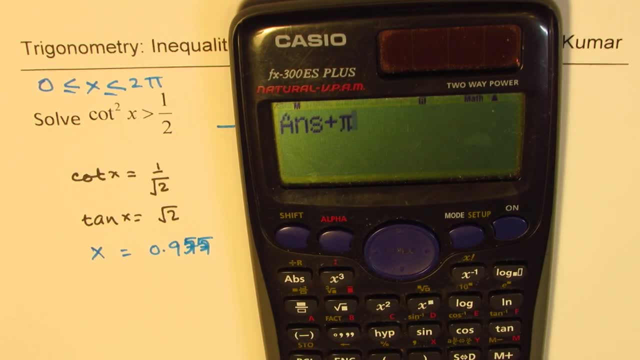 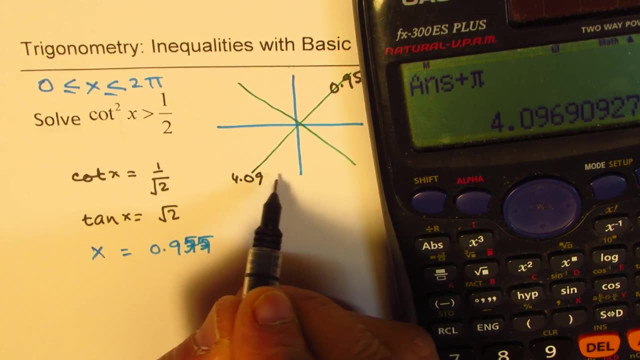 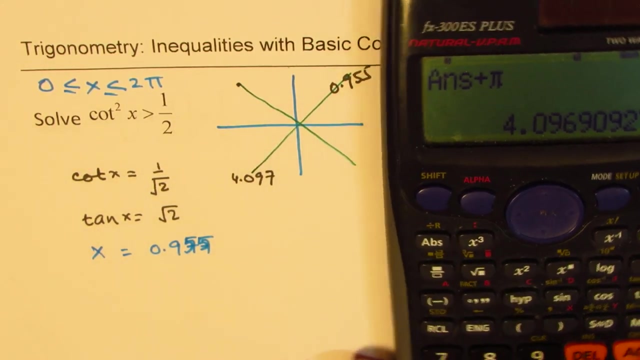 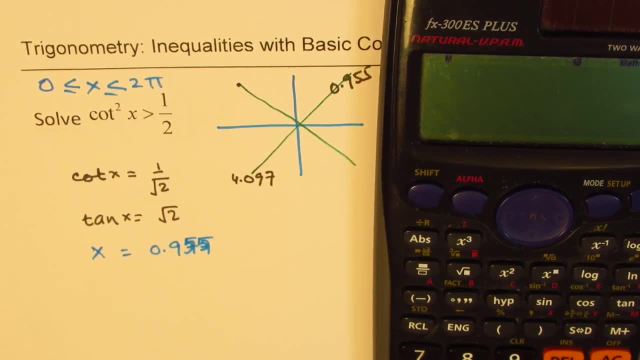 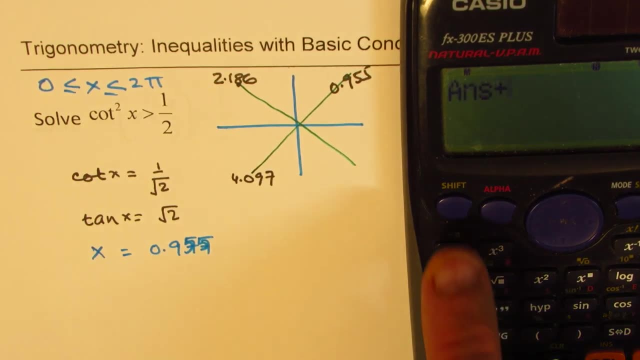 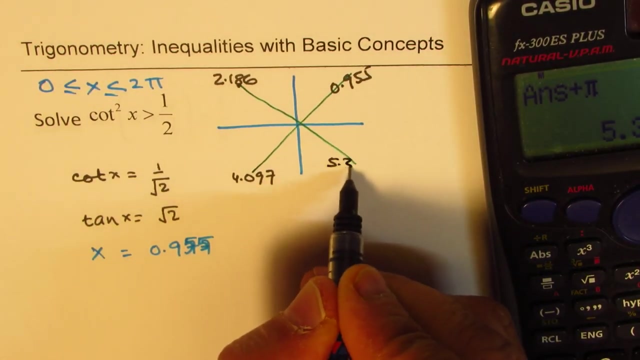 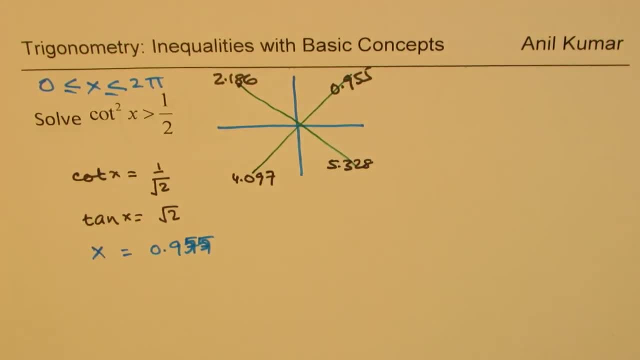 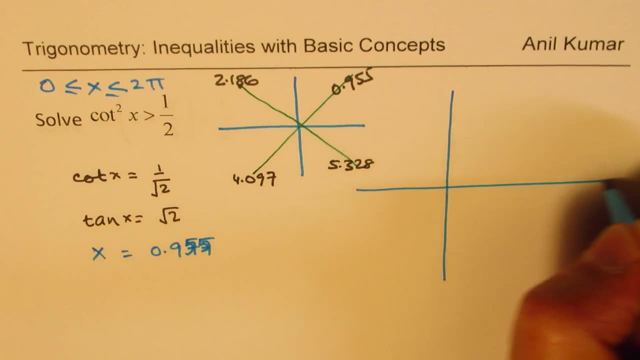 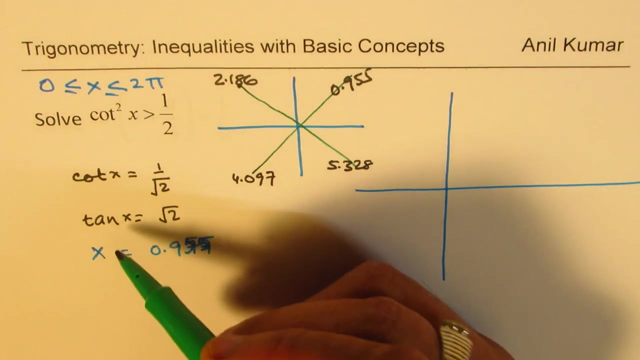 So we got our values. Now we know that the solution is somewhere close to these values. How do we figure out? For that? let us sketch the graph. Okay, So we are looking into cot square x, and that is our function. Now cot is reciprocal of tan. So the graph of cot. 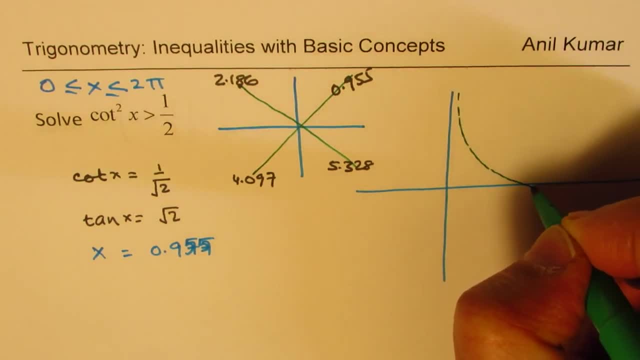 square x is kind of like this. So we will first sketch the graph of cot x. So what I am sketching here is not cot square x, but cot x. I am just making dotted graph, Okay. So I will just squeeze this. 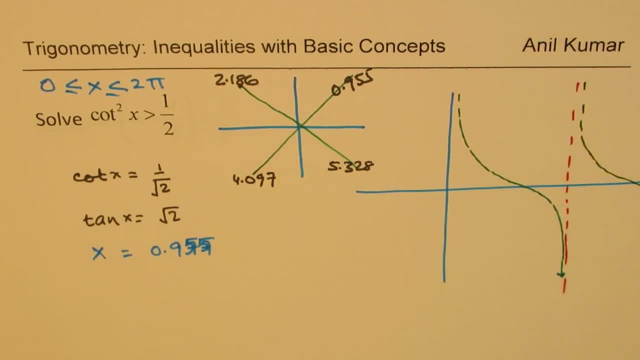 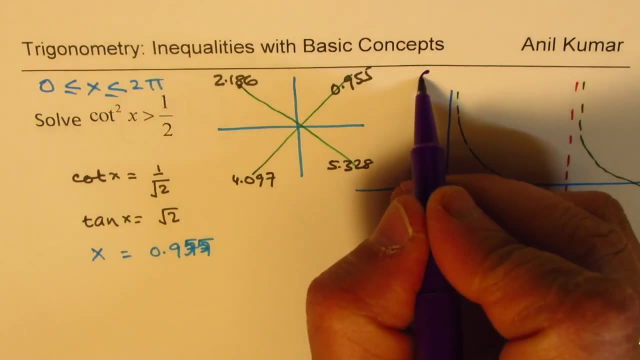 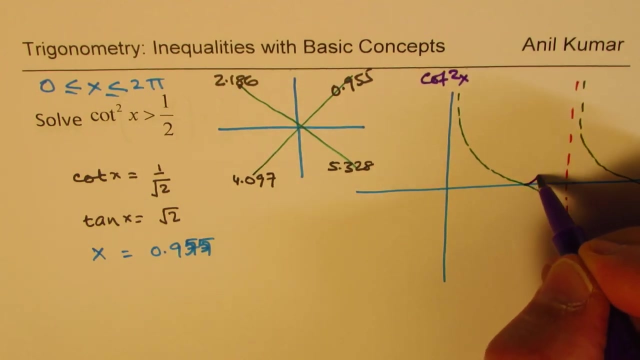 in into my page, but that gives you some sense of what it will be looking like. So if I want to make it cot square x, then everything is positive. So the portion which was negative will now be kind of like this: So this portion will be kind of like this: When we say that we 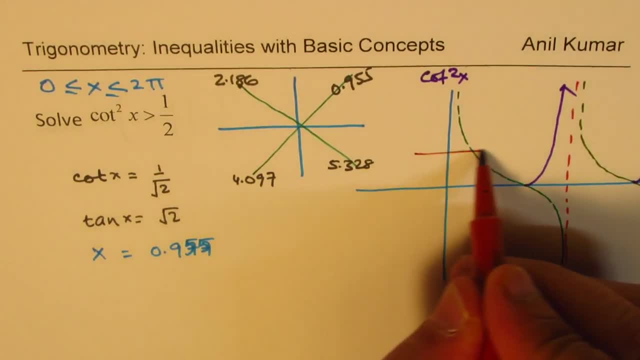 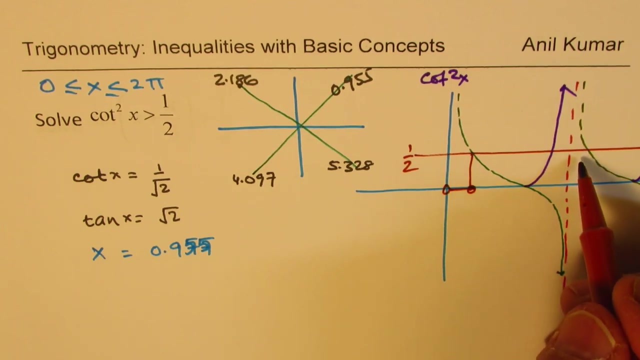 are looking for a value greater than half. so let's say: this is a line which says half. So everything above this is our solution. So we get a solution from here to here, right? So that is what all are, not. these boundaries are not included. So here to this place, right? 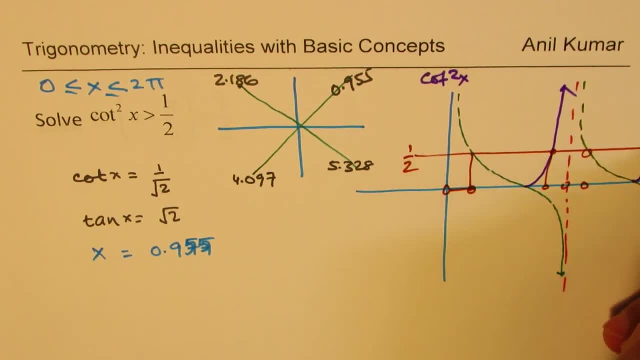 And then up to this place and then from here to this place, right? So these are the intervals which are included for us. Does it make sense to you? So, within 0 to 2 pi, those are our solutions. We already know what these points are. correct, Since we know these. 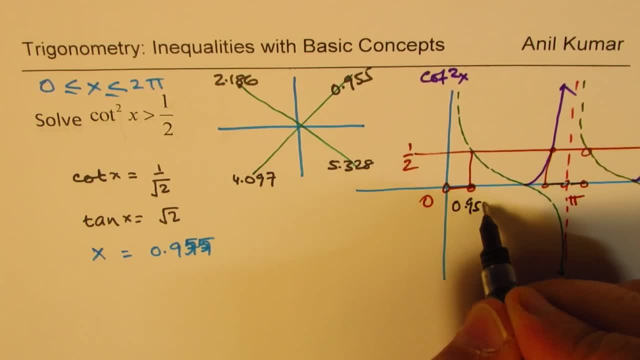 points, the first one here being 0.955,, then we have two points: this one, which is 2.186,, right, So this is what our solution is going to be. So, if this is a line, and then from here to this, point. then this is 2 pi. we have our solution. So we are going to have a solution of 0 to 2 pi. So, within 0 to 2 pi, we have a solution of 0 to 2 pi, then we have a solution of 0 to 2 pi, and then, from here to this one, 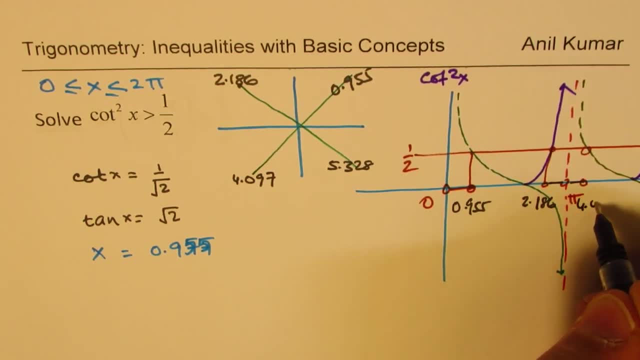 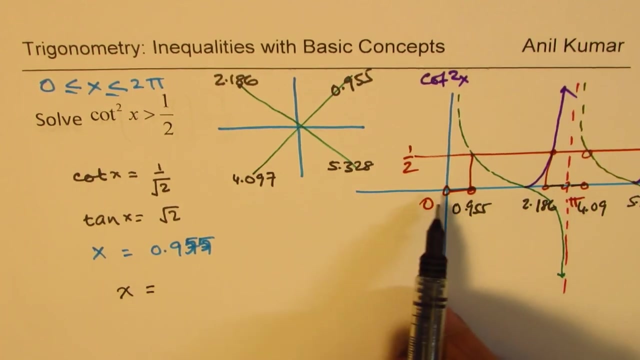 then here we have 4.097, and then we have 5.328, and that is 2 pi. So now you can write down the value for x, which is our solution, right? So these points should not be included. 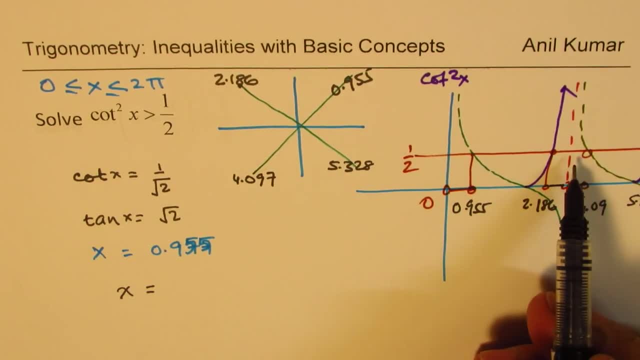 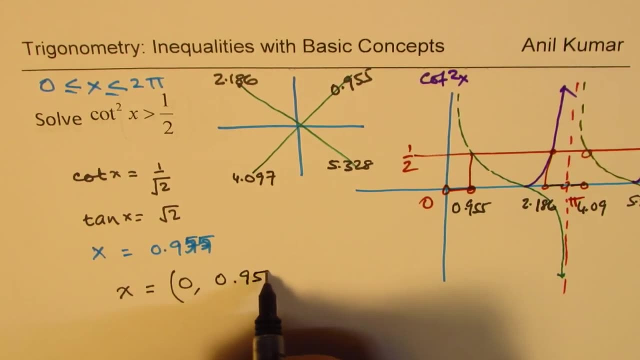 One, the inequality is greater than Second. there are points of discontinuity, correct. So from here we can write that the interval is from 0 to 0.955.. There's no need to write radians. Radiance is a ratio, right? So it doesn't really have a unit, okay, And then we have from: 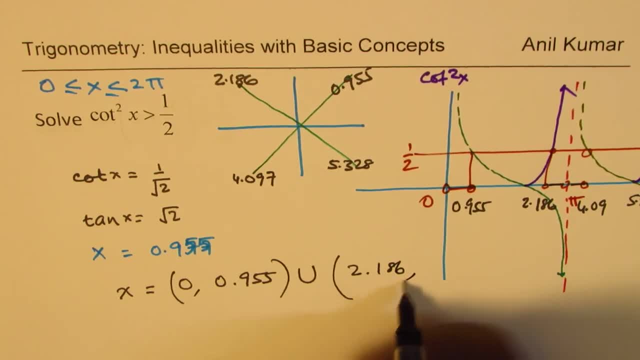 here to there, which is 2.186 to pi, and then we have from pi. You have to have this discontinuity because at pi cot x is not defined right. So 4.09 union, 5.32 to 2 pi. Is that clear to you? So that is how we are going to get the solution of this. 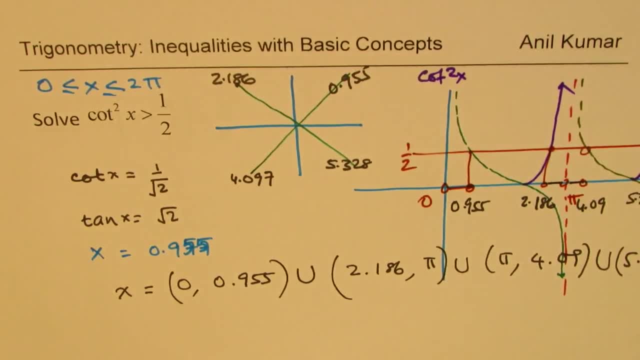 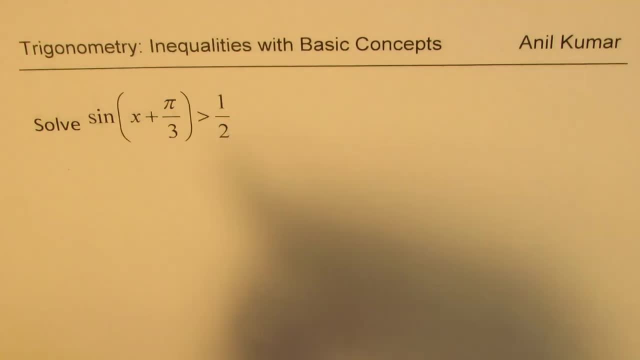 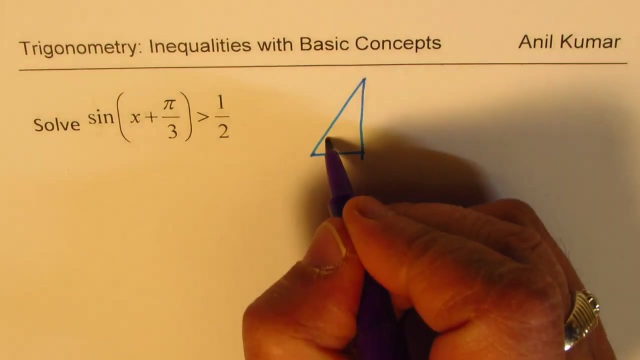 particular inequality. Perfect. Let's move on and take the other questions. Now we have sine of x plus pi by 3, equal to half. Now when is sine theta half? Let's say this angle here is theta for us, So sine theta is half. when 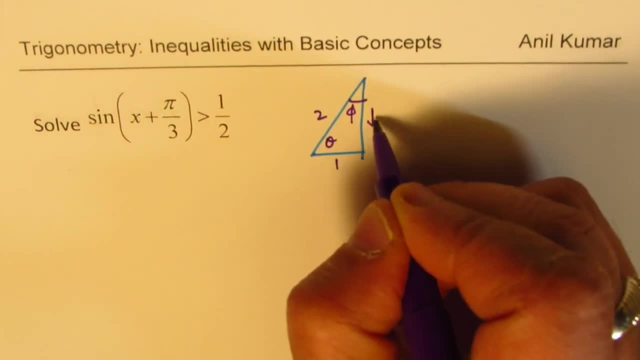 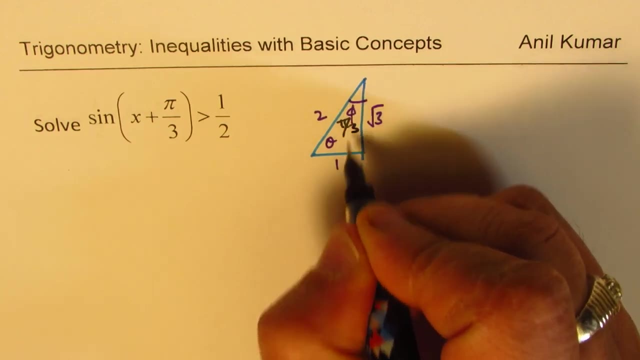 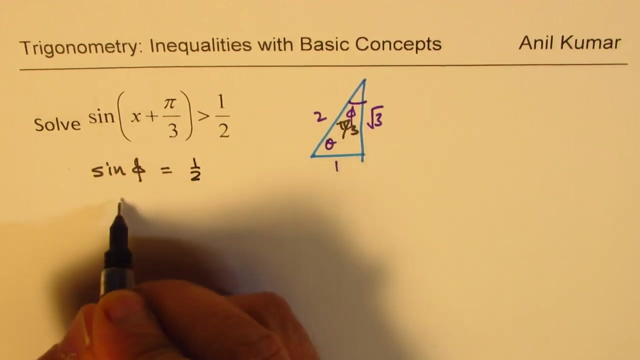 well, for this angle it is half, right, Not that? okay. So that angle it is half and this angle should be pi by 3.. So we know, sine theta, let me write phi now. sine phi is equal to half when the angle phi is pi by 3.. 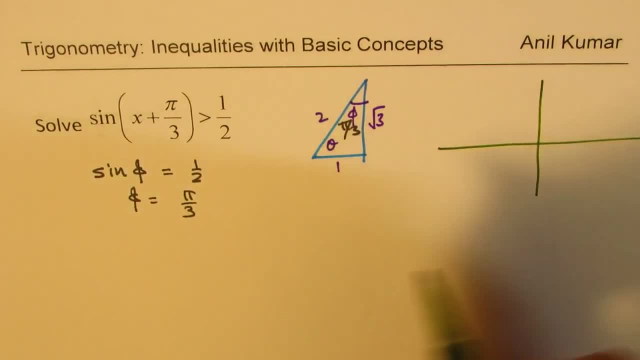 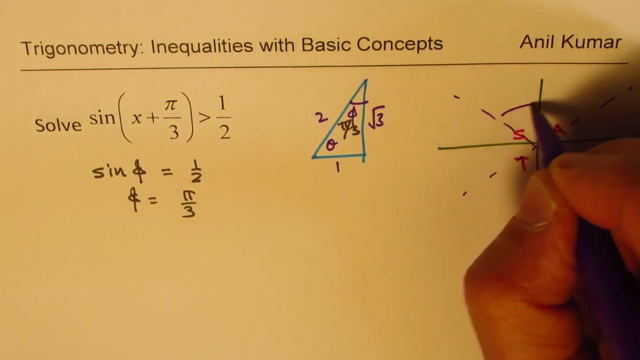 Now we are interested in finding a solution when it is greater than half. Now, sine, you know, a positive is, sine is positive in second quadrant, right. So we know one thing: that in our case it is going to be greater than half between these two values. right there, correct? 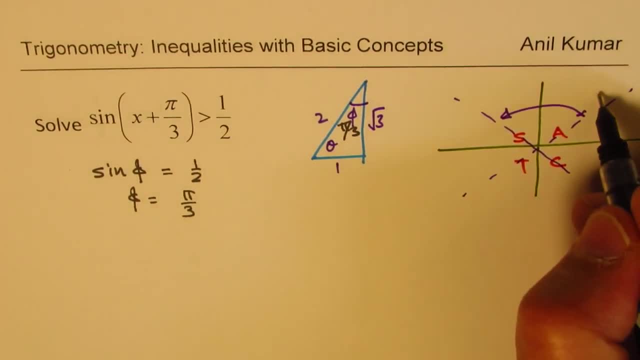 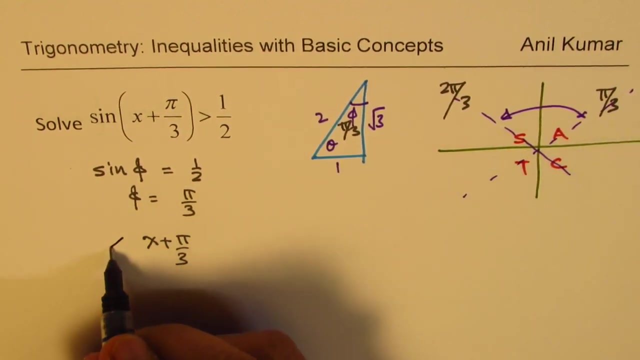 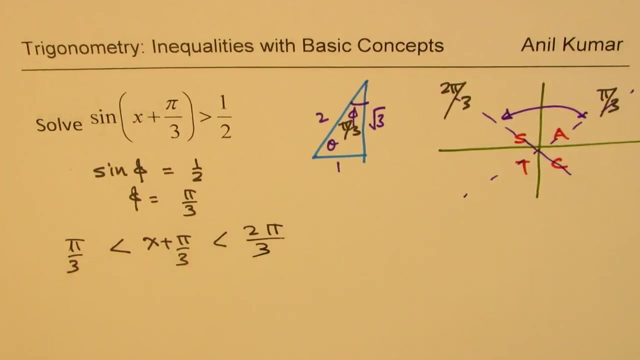 So from the given equation, since we know this is pi by 3, the other one is 2 pi by 3 when it is equal to half, correct? So the solution becomes that x plus pi by 3 should be greater than pi by 3 and should be less than 2 pi by 3, clear. 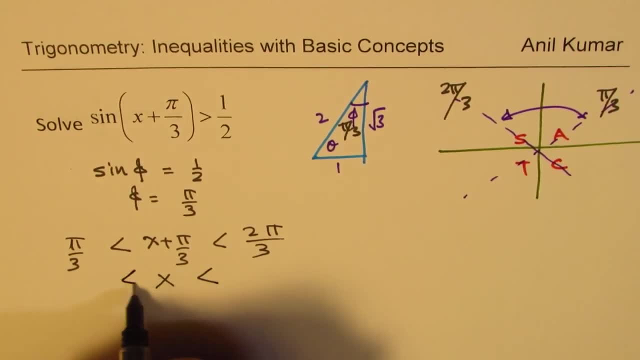 So what should happen to x? To get the value of x, we have to subtract pi by 3, right? So we have pi by 3 minus pi by 3 and 2 pi by 3 minus pi by 3.. So that gives you the solution for x. 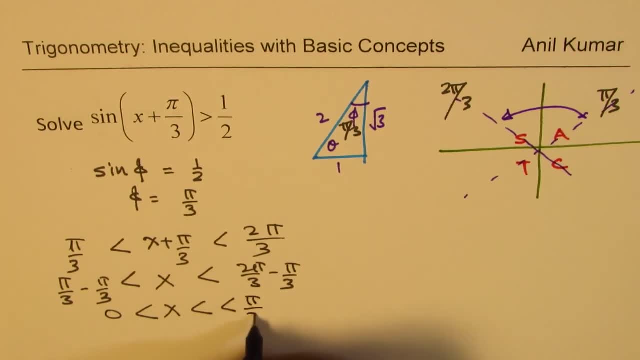 which should be greater than pi by 3.. So we have pi by 3 minus pi by 3 and 2 pi by 3 minus pi by 3.. So in this case x should be greater than 0 and less than pi by 3, correct, So that becomes our solution for the given equation. 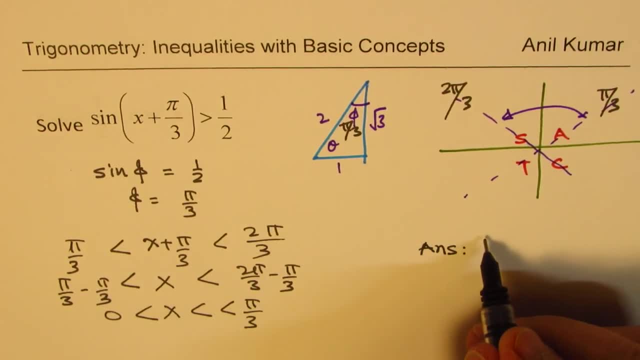 So remember this. So the answer here will be from 0 to pi by 3, correct, Licensed. Now let's take two equations, forksen, and multiply them with the Videos. We, since we, are writing in this form, all our solution. I've rewritten the solution instead of inequalities. 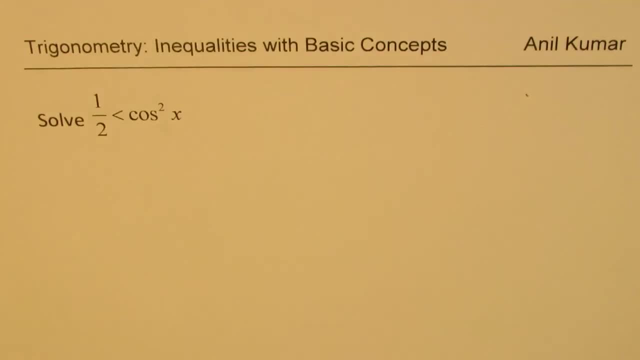 in the interval notation. Is that clear to you? The next question here is: cos square x2 f is greater than half. How much is cos square x2 f divided by one? You see it is actually 4 times the real value for cos times infinity, x1 and 0.. 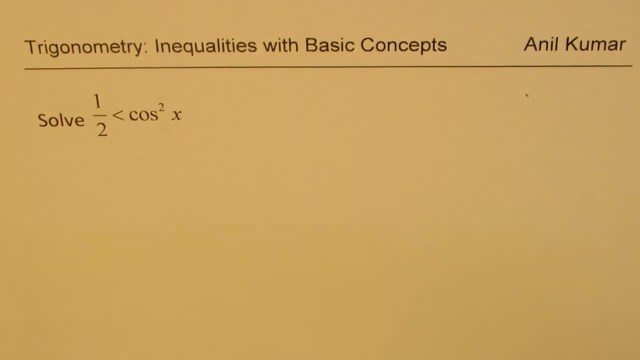 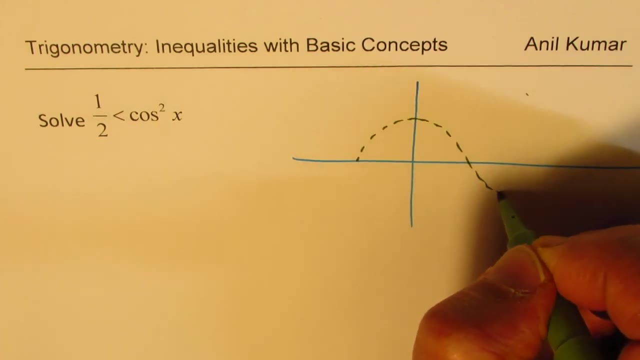 than half right. So, okay, let us quickly sketch and then solve, right? So we have cos x function which will be kind of like this: We are working in 0 to 2 pi. The square x function will always. 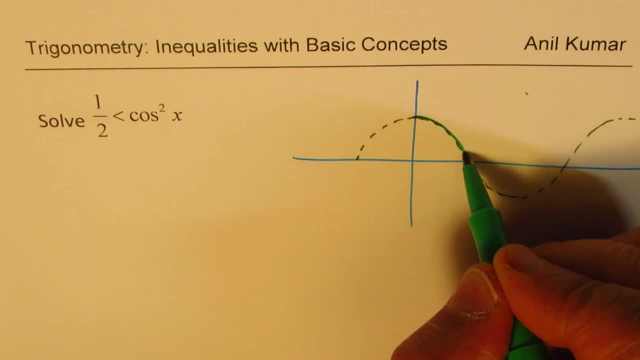 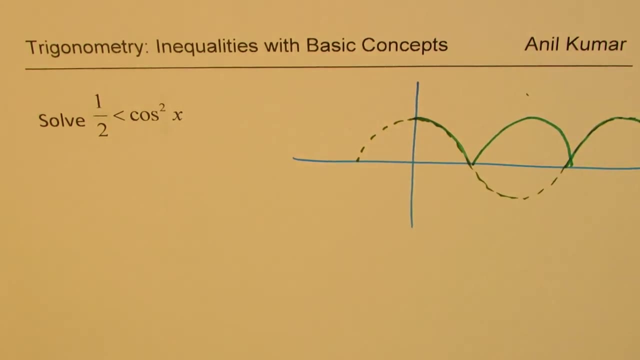 be positive: never more than 1, right, something like this: okay. And here again it is going to be like this: okay. Here it will be kind of like this, Not really over it, but as far as the inequalities are concerned, we could consider that to be okay, right? So what you need to. 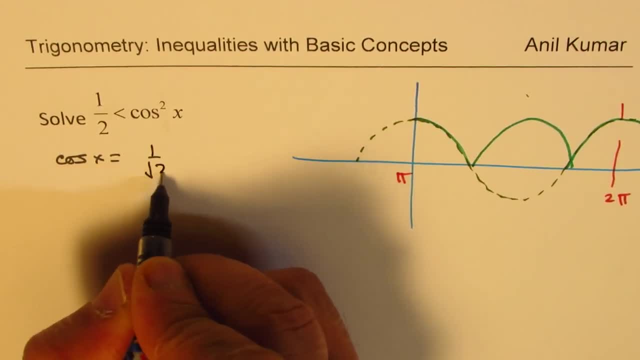 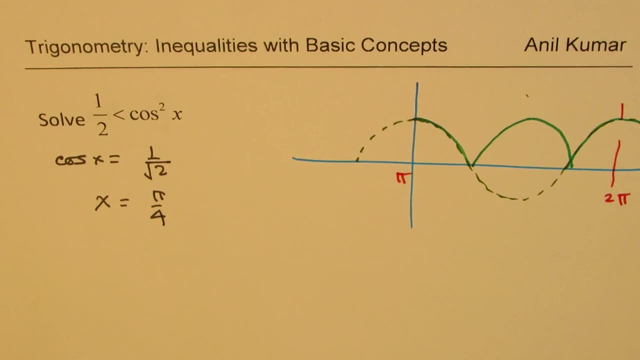 work out is: when is cos x equals to 1 over square root of 2.. That is what we need to find, And that is when x is equal to pi by 4, correct. Now getting back to our quadrants, we know cos is. 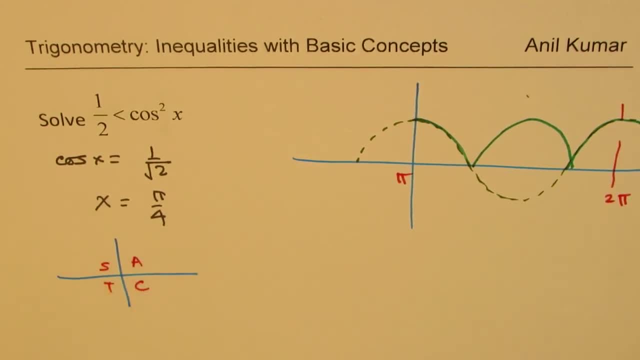 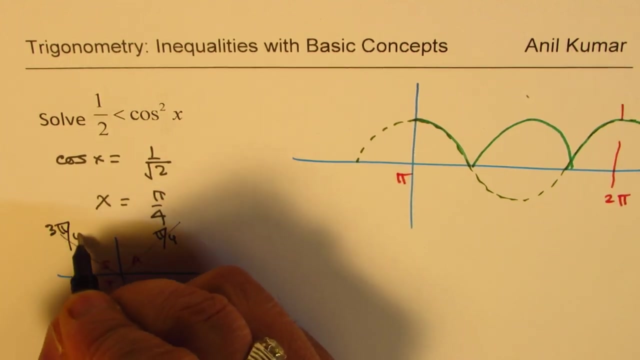 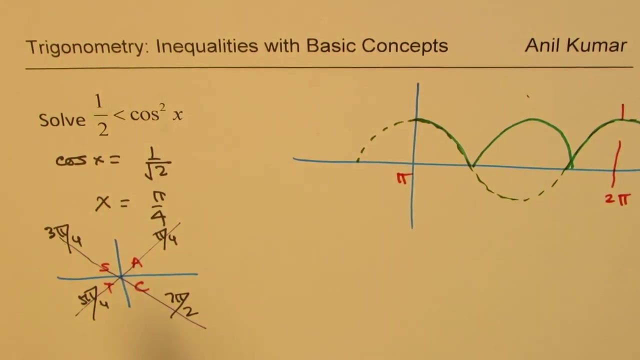 positive. All are positive here, sine tan and cos. Now, the cos is positive in which intervals in first and fourth quadrant, right. So what we have here is pi by 4, 3, pi by 4, 5, pi by 4 and 7, pi by 4, right. These are the values at which cos square x is equal to 1 over. 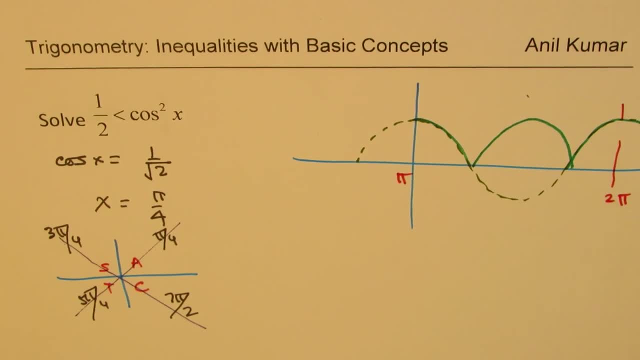 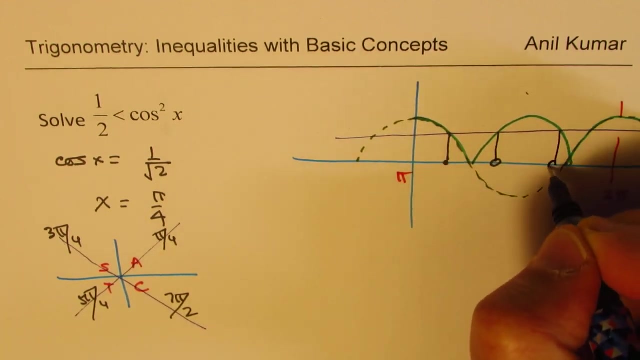 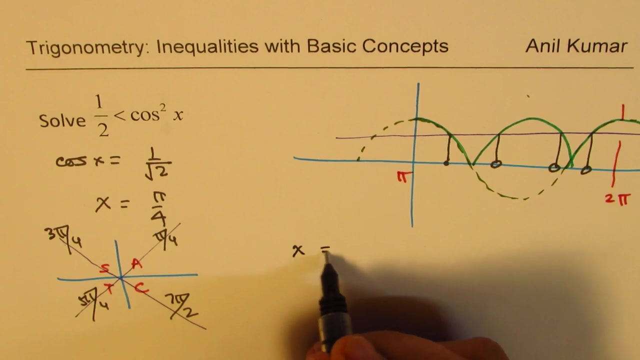 2 cos square x, So both negative and positive will be taken. We want these values greater than say we sketch it like this: We know these values, We know these values, correct, Perfect, So greater than means. from here you can see our answer for x is: we are not equal to right. So 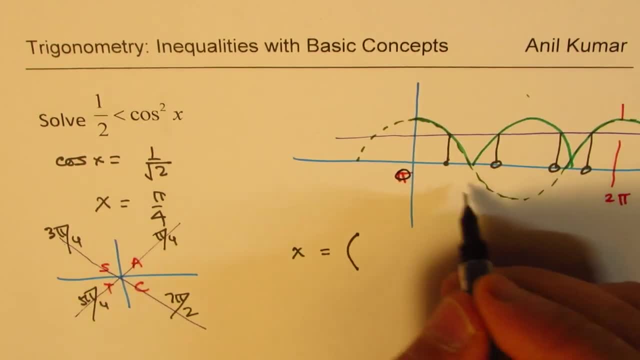 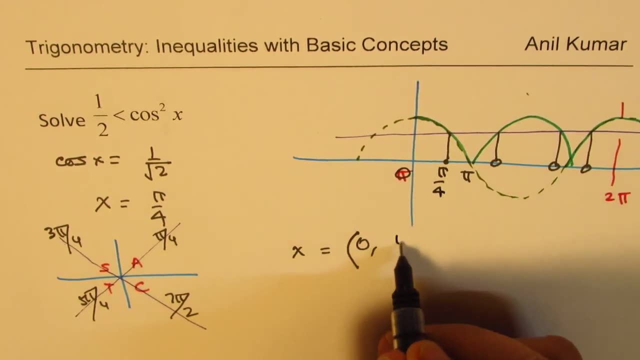 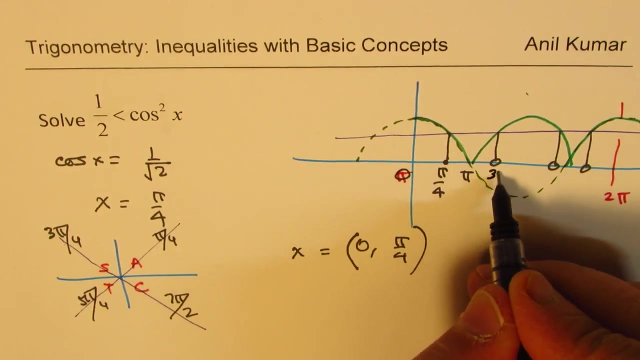 we will not include 0. I mean this should be 0,. okay, This is pi. So from 0 to the first regressor of this side, its norm. you can see I am using 3 minus 4 pi by 3,, 5 pi by 4,. 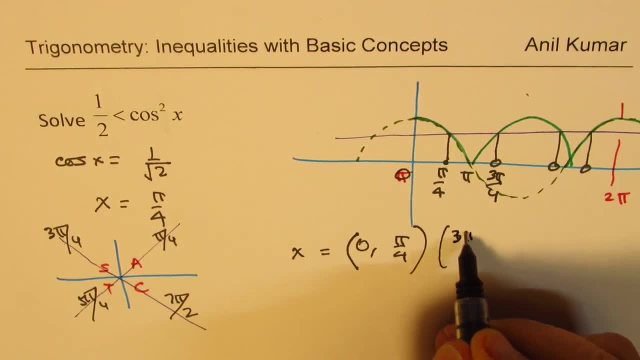 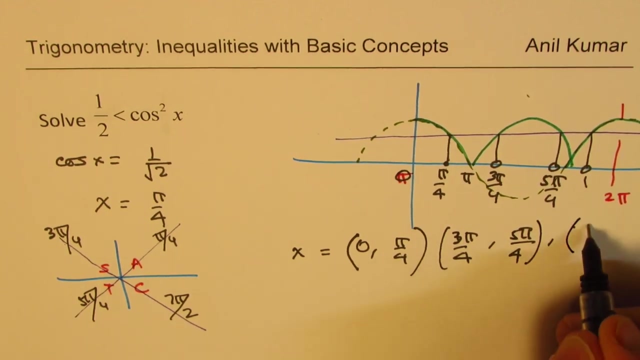 fine, So by not today any more than 5 times STR. so it will be equal to 1 point over 9, omega 0.. There it goes down, And then again it is up when it is 3 pi by 4, St들. 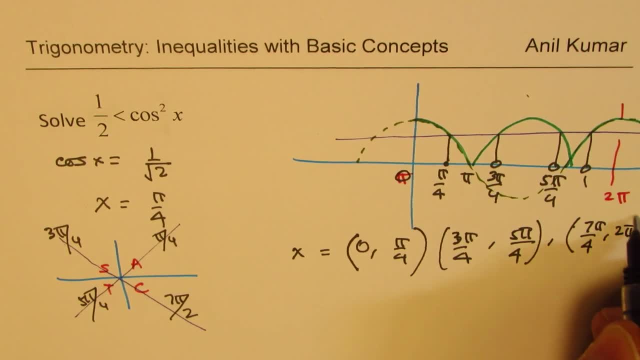 db. p length 0 to 5, lambda 0.. Up to 5 pi by 4.. St Br': 1. St Br'- 1. St Br' 5write' Santa455.. St Br'- 5write Santa455.. 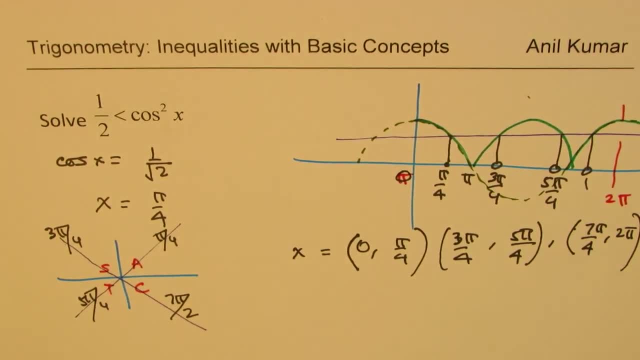 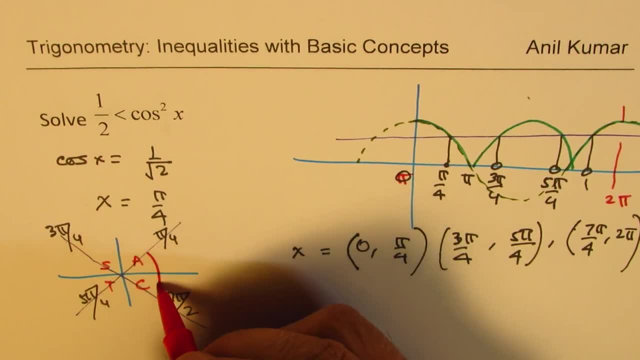 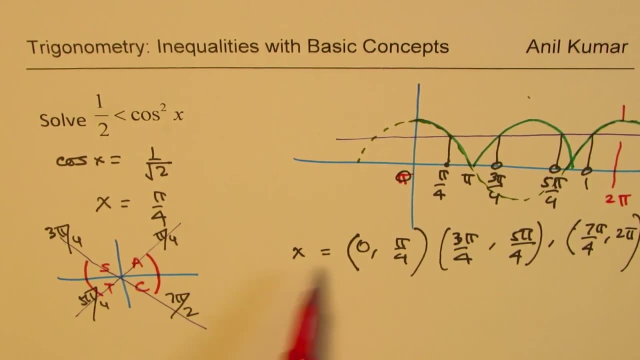 square x is greater than half when it is closer to this portion. Is it okay? Does it make sense? So that is how you could visualize and get your answer. So I hope this concept of using the graph and the coordinates where one is positive or negative, and just finding 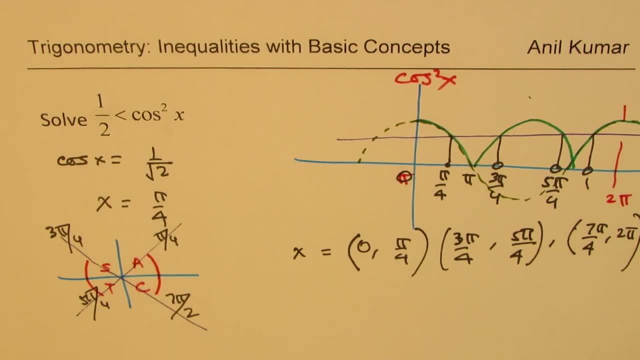 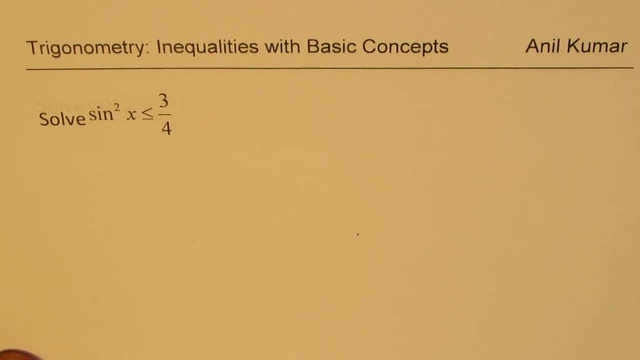 one value when it is equal to the given thing helps to solve trigonometric inequalities. Perfect, Now the last question here, almost the last question, one more to go. I will leave this for you, right? So we did cos square x. Now you can do sin square x. write down. 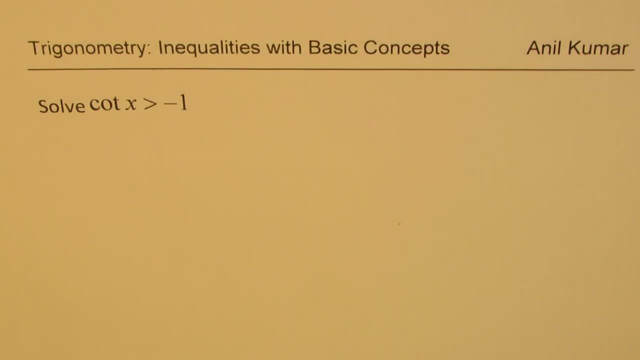 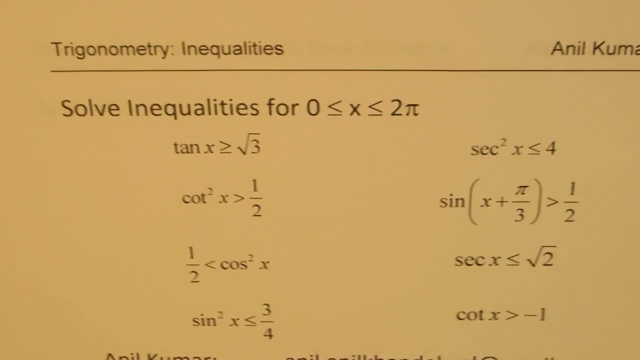 your answer follow a similar method. And also the last question, which is cot x greater than minus one. So I'll leave that for you to do. Try to solve these questions And I hope you find it interesting and useful. Now we have actually practically solved all. 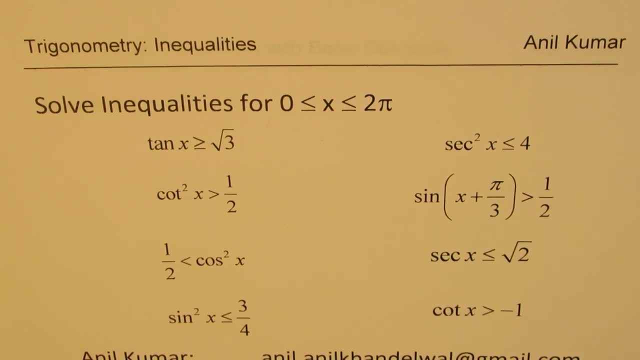 these questions. In case you have any doubts, you can always email me. You can also provide me with your answers, So I hope that works. Feel free to make suggestions, write your comments and share your questions. Let me again thank Mr Kapil for sharing this particular question: All the best.